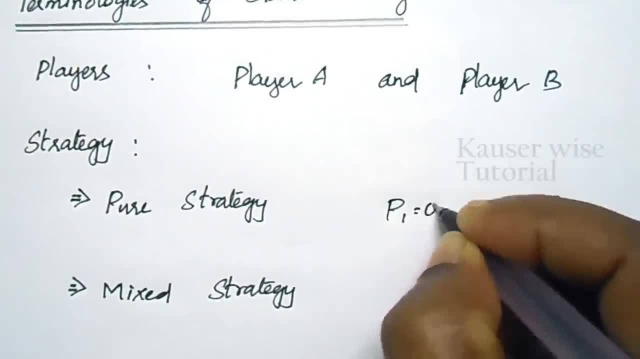 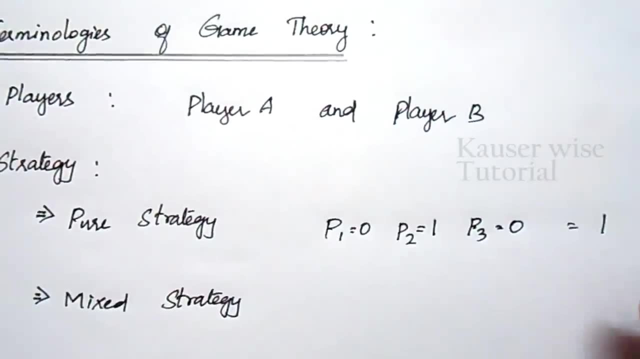 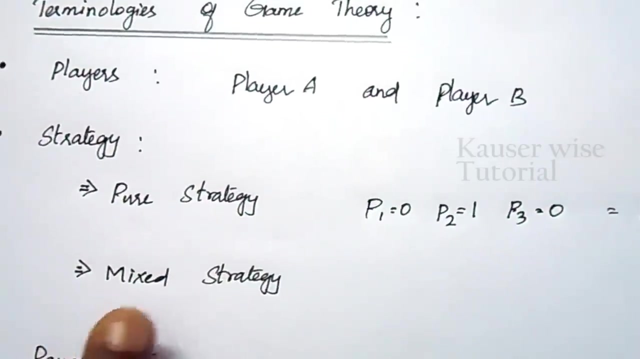 So the probability is one. The remaining two strategy probability is zero. So what is the total? 0 plus one plus zero is equal to one. So the sum of these probability is one. This is called as pure strategy. So let me explain mixer strategy. Mixer strategy means if a player follows more than one. 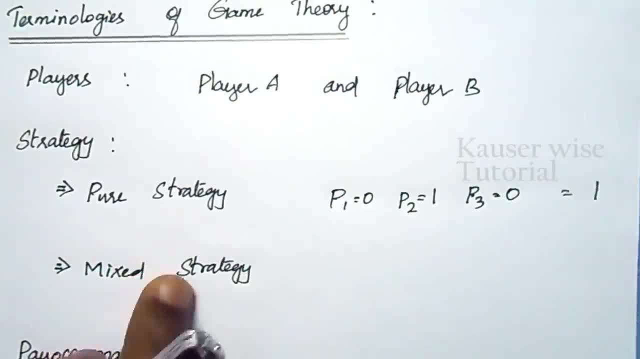 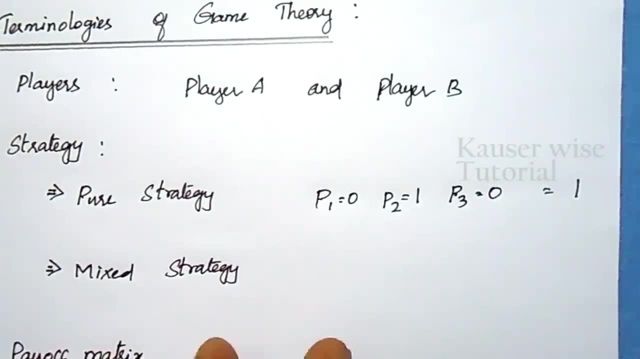 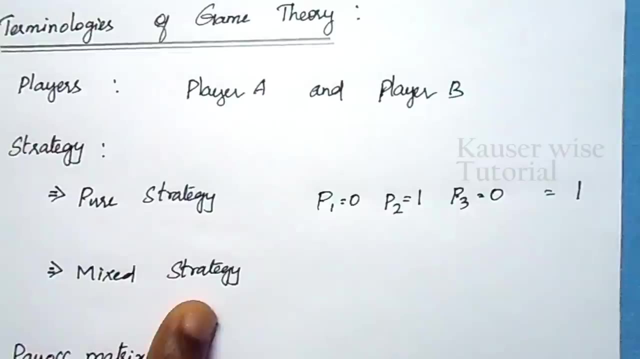 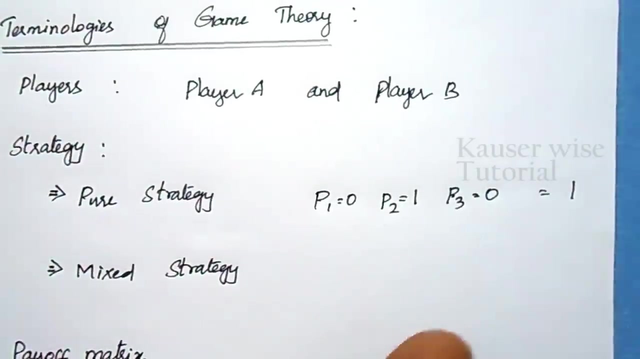 strategy, then the player is set to follow mixer strategy. See here, Probability of the selection of a particular or individual strategy will be less than 1.. Why? Because here the player will select more than one strategy. So the sum of the total probability will be 1, but each probability value will be less than 1.. 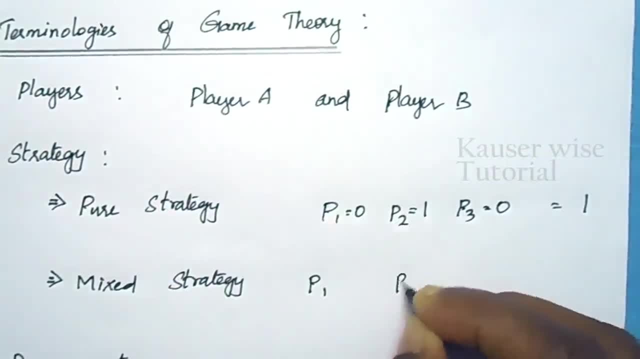 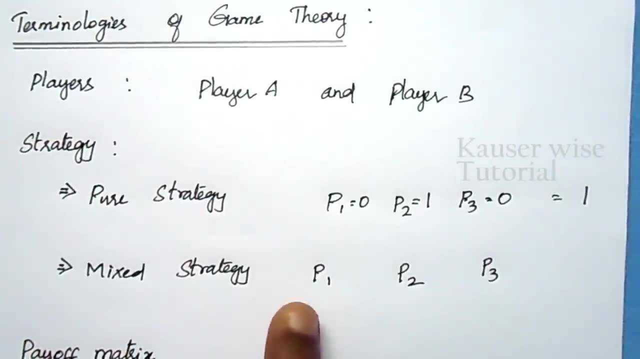 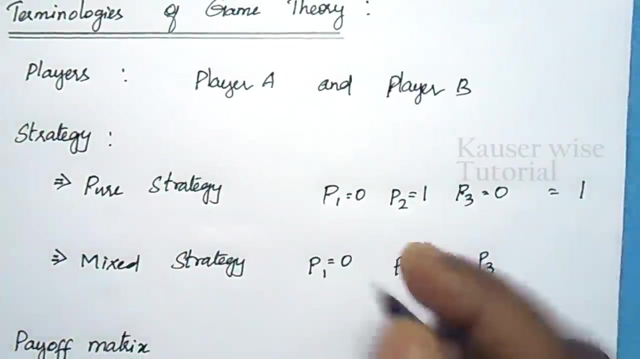 Let me show if we have 3 strategies: P1, P2 and P3.. A player is going to select more than one strategy, So let me take strategy 1 and strategy 2.. Each strategy value, the probability value will be less than 1.. 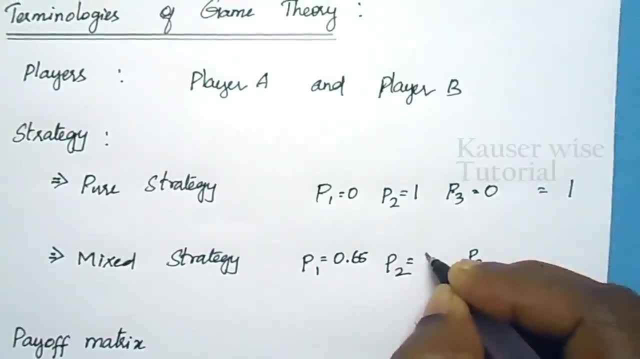 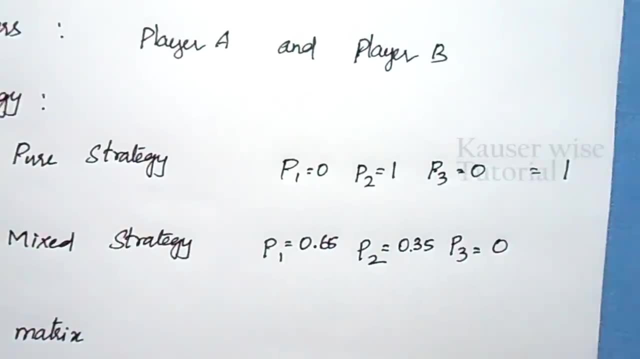 For example, 0.65, and second one is 0.35.. The third one is 0.. What is the total? The sum will be is equal to 1, only 0.65 plus 0.35 plus 0 is equal to 1.. 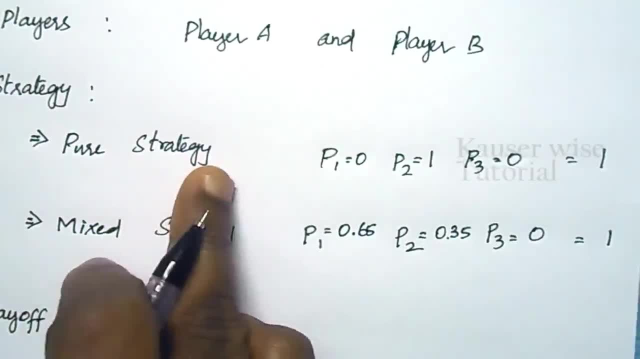 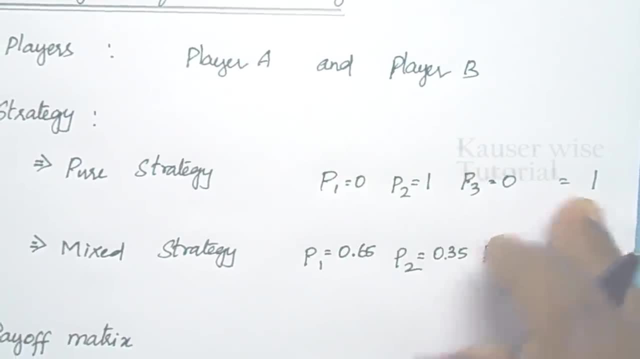 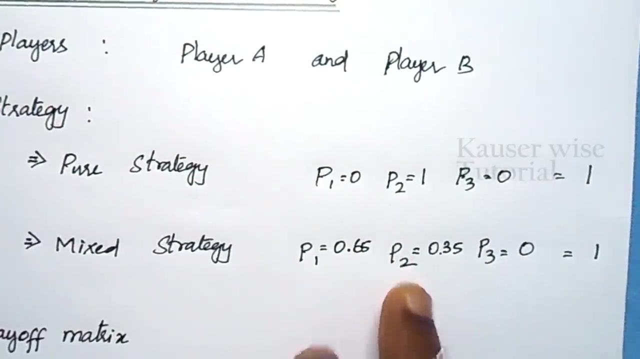 So this is called as mixer strategy. Pure strategy means a player will select Only one particular strategy. The probability value will be 1, total also 1 because he ignoring the remaining strategies. Mixer strategy means the player will follow more than one strategies. 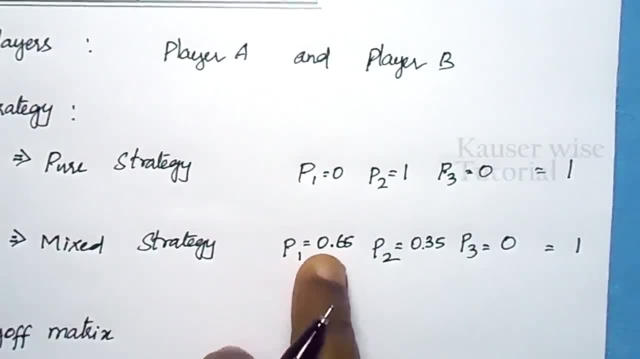 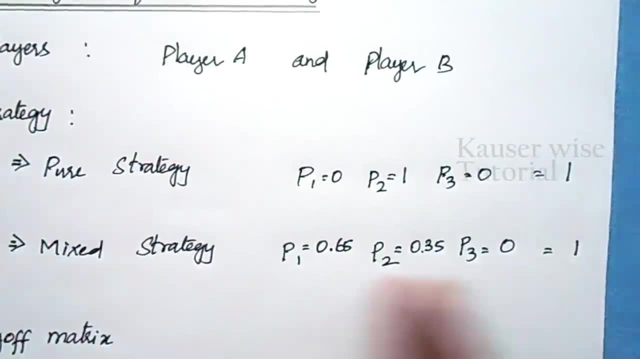 OK, but the each strategy probability will be less than 1, but the total will be 1.. This is called as mixer strategy. We will see this in detail along with the problem See. the next one is payoff matrix. Look at the sample payoff matrix here. 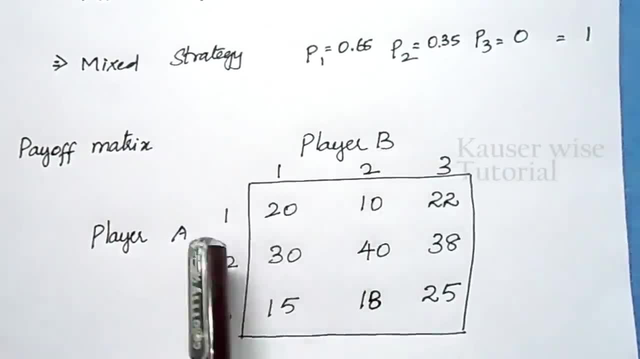 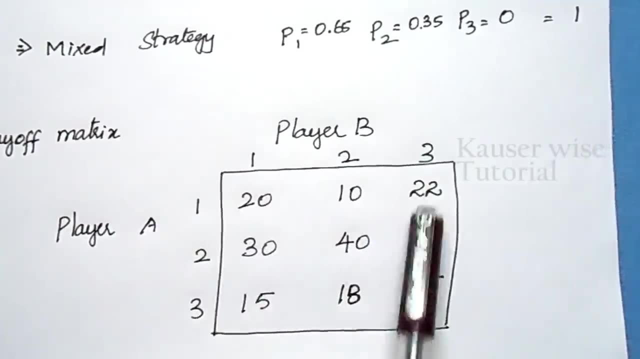 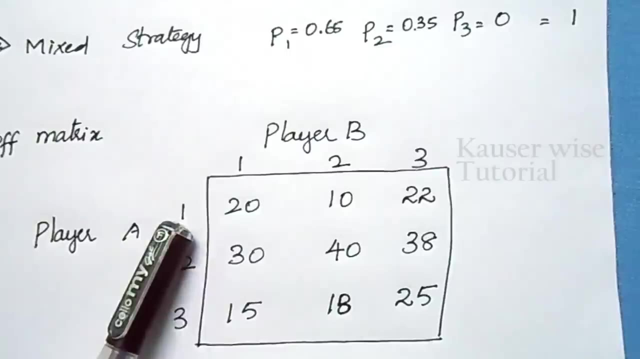 We have two players- player A and player B- and here we have three strategies: one, two and three, Player B also having three strategies: one, two and three. So these are the outcome of the different combination. See, if player A select the first strategy and if player B select the second strategy, the outcome will be 10.. 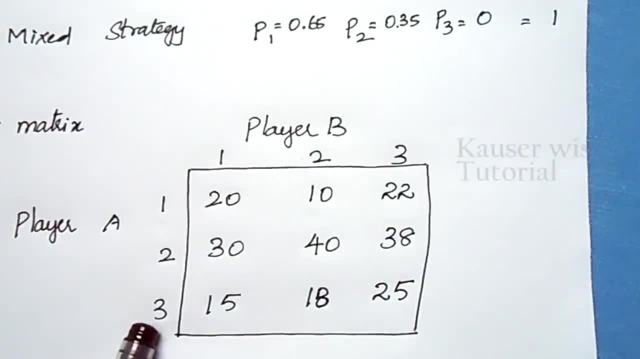 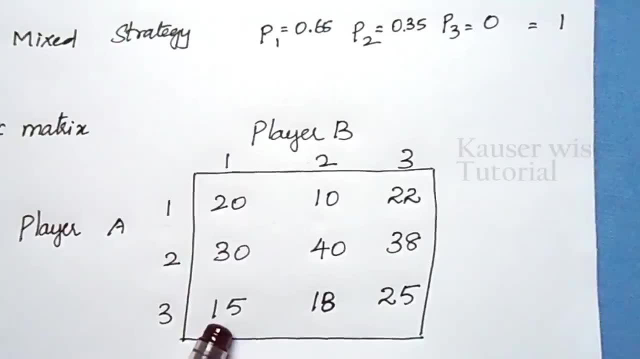 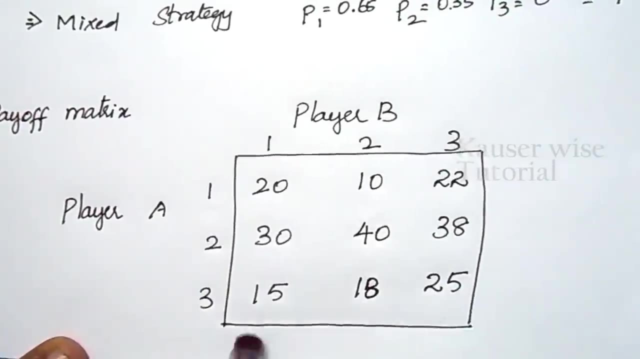 OK, and if the player A select the third strategy and player B select the first strategy, then the combination- That is the outcome- will be this, that is, 15.. OK, these are the outcome of different combinations. OK, see, if the outcome is positive means then it is a gain to player A and loss to player B. 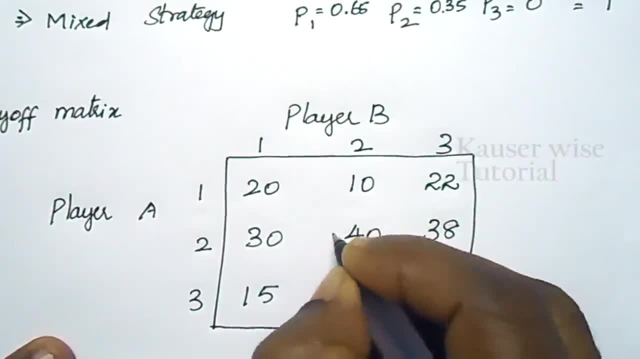 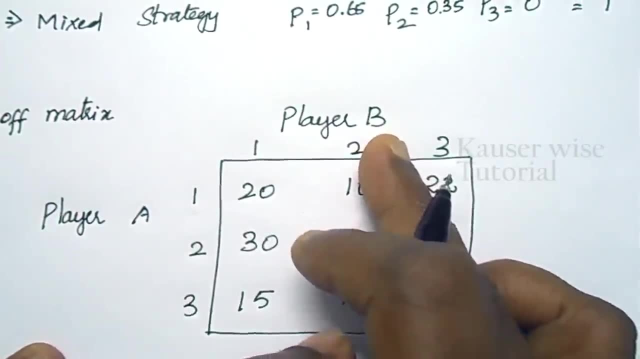 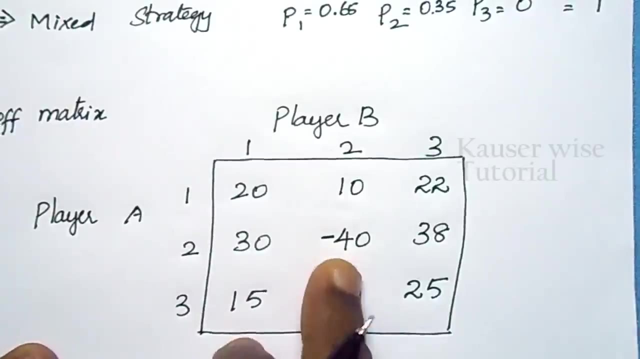 OK if we get any negative value, for example minus 40. If player A select the second strategy and player B also follows the second strategy, then the outcome is minus 40. Which means player A gets loss and the same amount will be gained to player B. 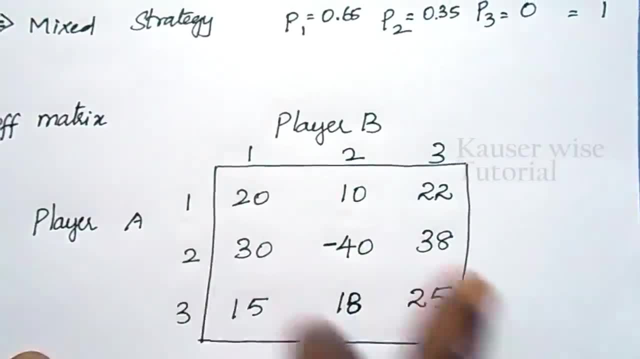 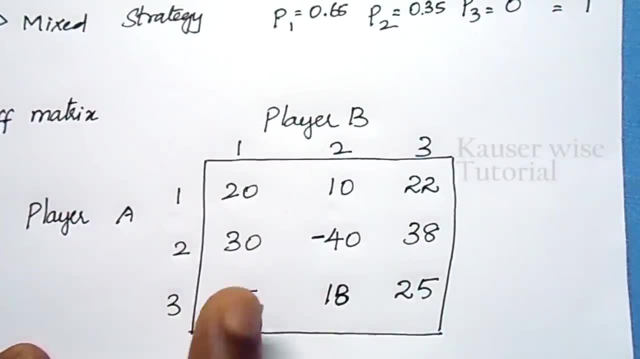 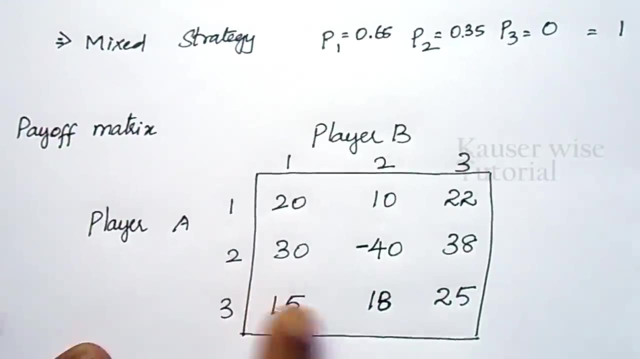 OK. again, I repeat: if the outcome is positive means then it is gain to player A and loss to player B. If we get any negative outcome, then it is a loss to player A and gain to player B. OK, this is called as payoff matrix. 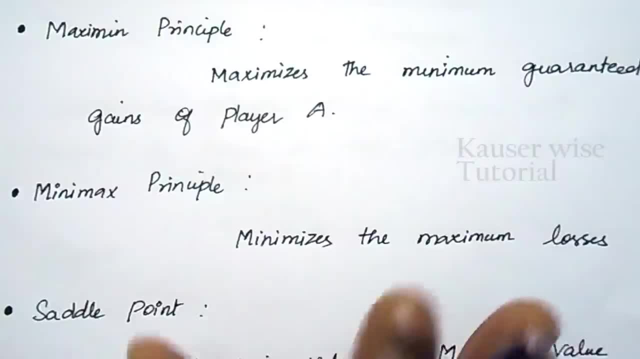 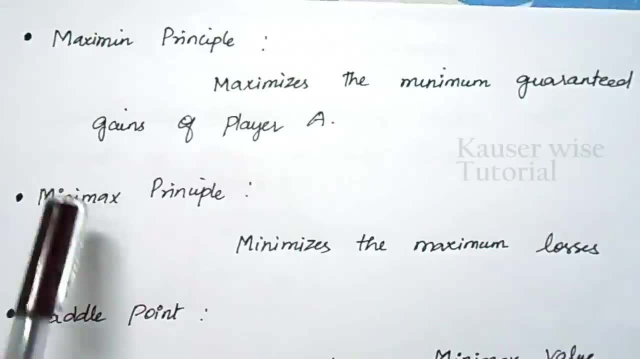 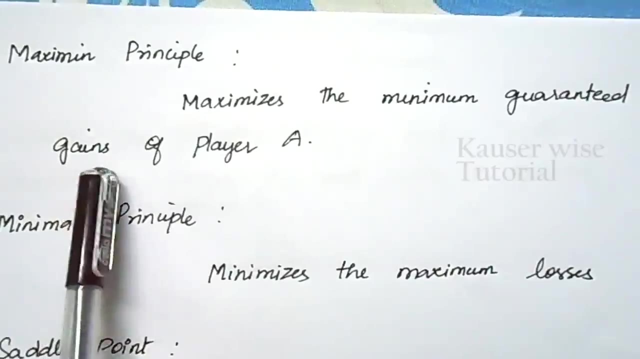 This is only example. OK, now let us see the next one. The next one is maximum principle. See, in game theory there are two principles. One is maximum, The other one is minimax. Maximum principle means maximize the minimum guaranteed gain of player A. 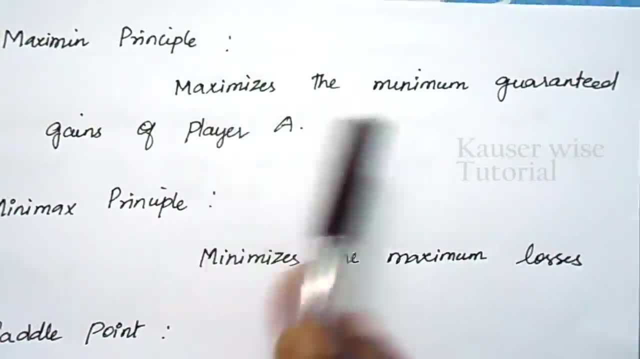 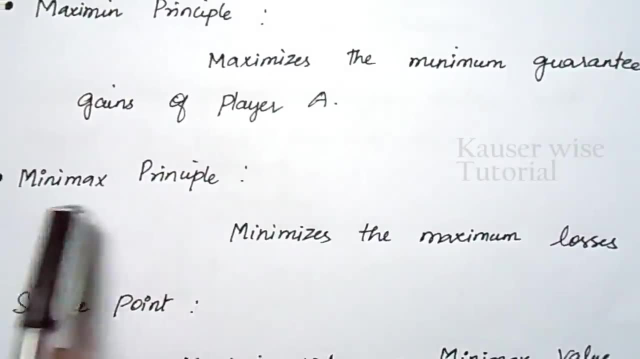 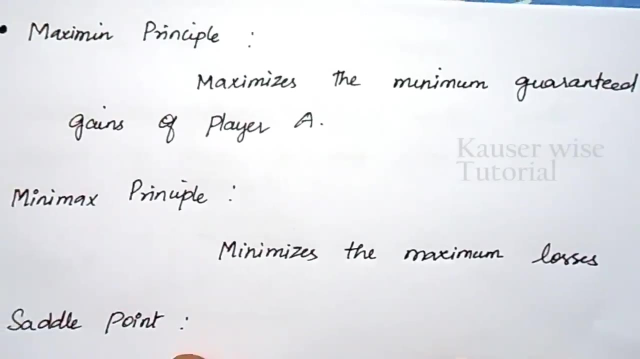 OK, the ultimate objective is to maximize the minimum guaranteed gain, So this principle is called maximum principle. OK, the next one is minimax principle. Minimax principle means minimizes the maximum losses. OK, The ultimate objective is either to maximize the minimum gain and minimize the maximum loss. 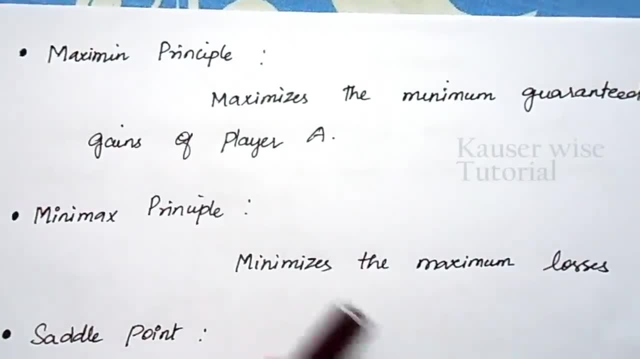 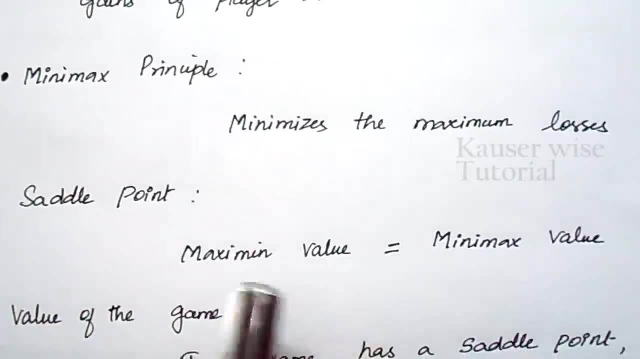 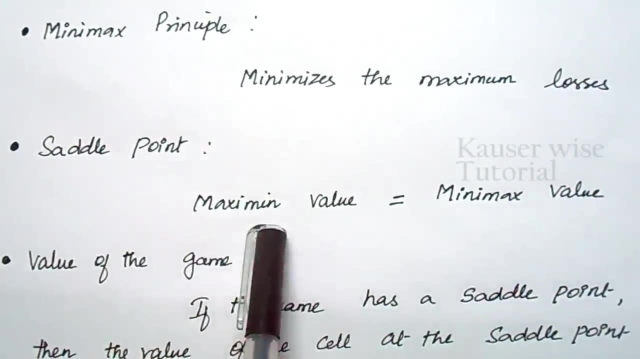 These are the two principles which we follow in the game theory. We will see this in detail along with the problem. The next one is saddle point. Saddle point means where the maximum value is equal to minimax value. Then the game will have saddle point. 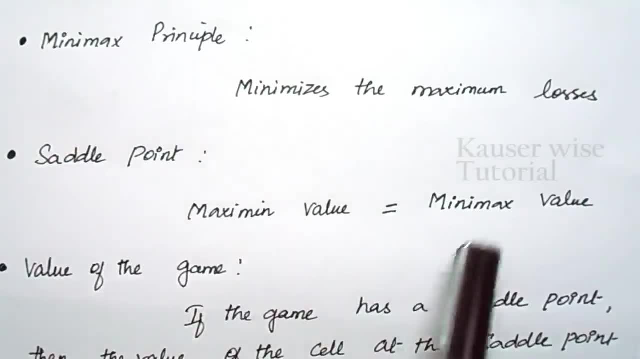 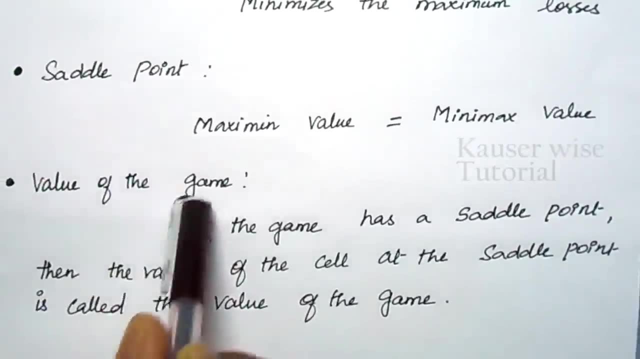 The intersecting point will be equal. That is the maximum value. Minimax value will be equal. Then the game will have saddle point. OK, the next one: value of the game. Value of the game means if the game has a saddle point. 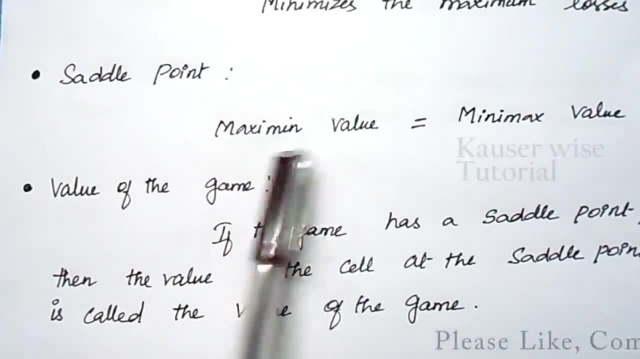 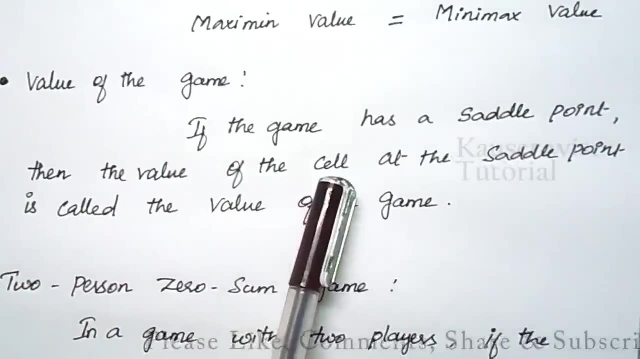 I told you know, saddle point means where the maximum value is equal to minimax value. OK, if the game has a saddle point, then the value of the cell at the saddle point is called value of the game. That is the intersecting point. 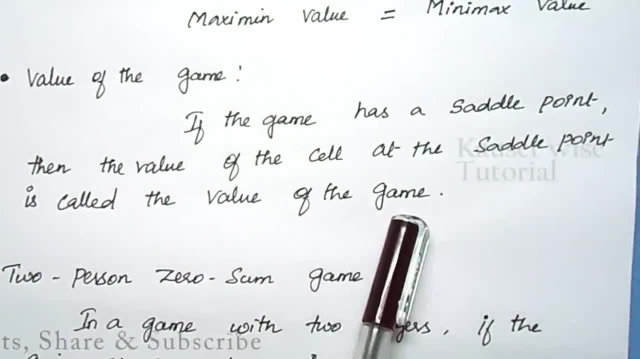 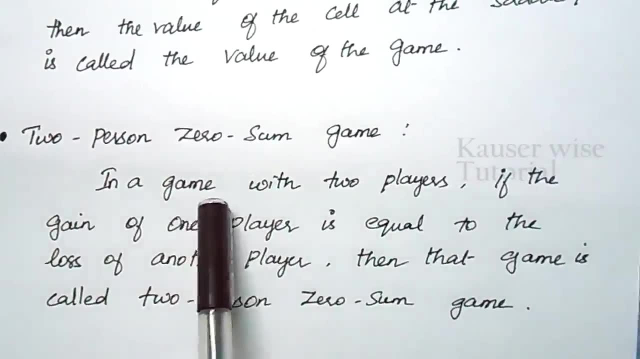 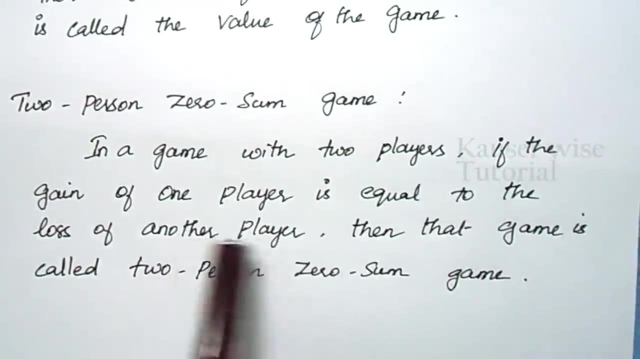 The value. The outcome is called value of the game. OK, the last one is two person zero sum game. OK, two person zero sum game means in a game with two players, if the gain of one player is equal to the loss of another player. 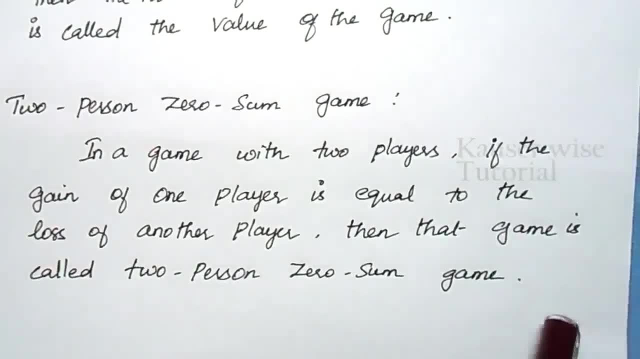 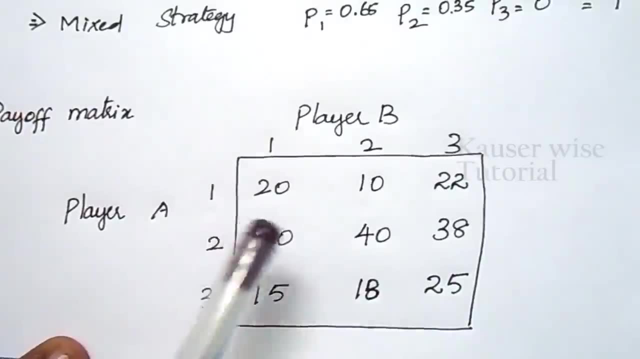 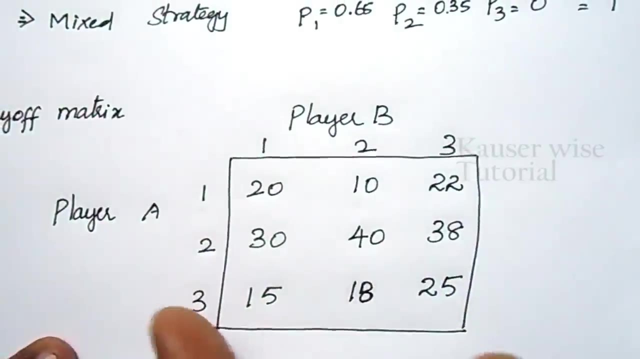 then that game is called two person zero sum game. For better understanding, see the payoff matrix. See: if the outcome is positive means then it is a gain To player A and loss to player B. OK, if we get any negative value, for example minus 40,. 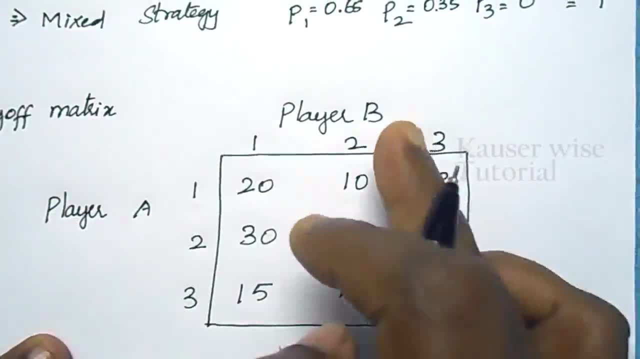 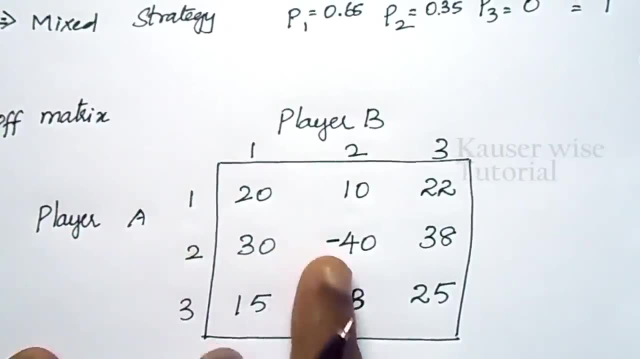 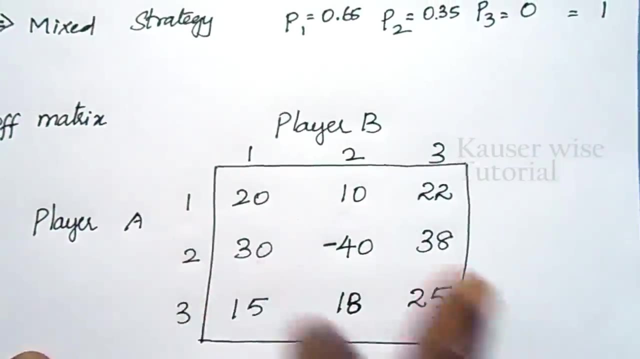 if player A select the second strategy and player B also follows the second strategy, then the outcome is minus 40, which means player A gets loss And the same amount will be gained to player B. OK, again, I repeat: if the outcome is positive means then it is gained to player. 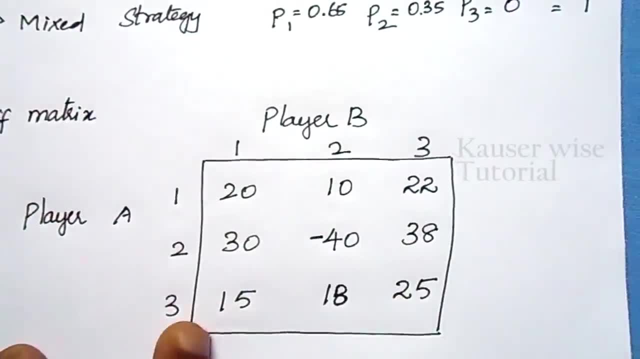 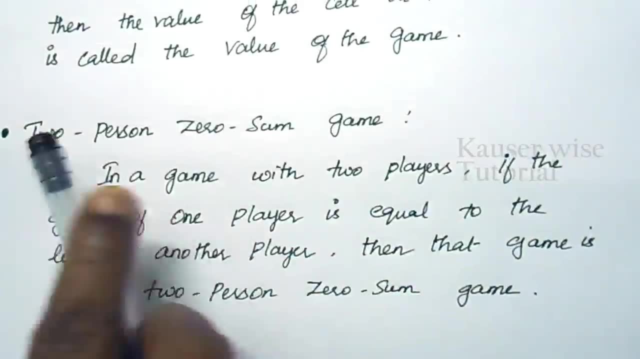 A and loss to player B. If we get any negative outcome, then it is a loss to player A and gain to player B. OK, this is called as two person zero sum game. OK, so far we have discussed the basic terminologies of game theory. 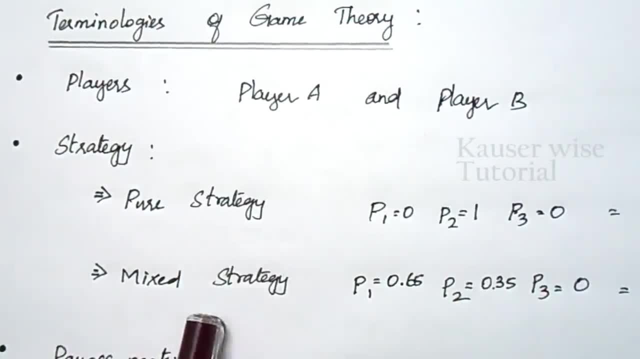 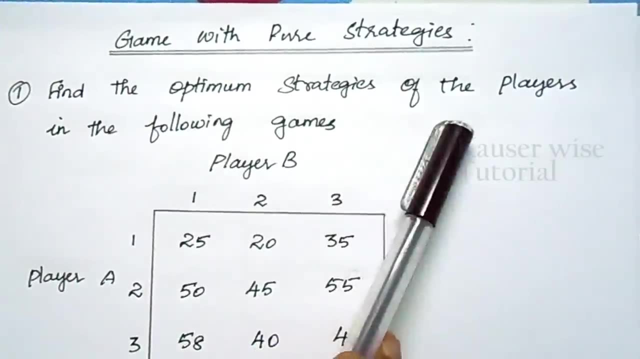 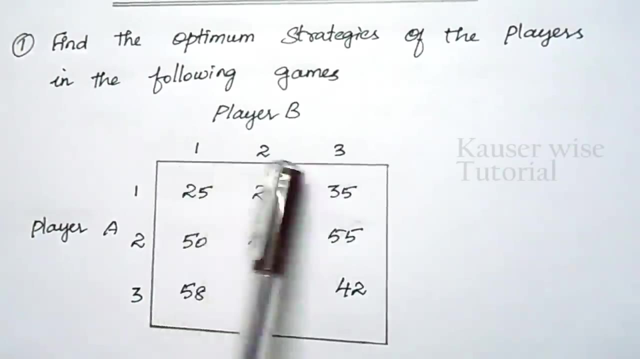 Now let us see the problem for pure strategy and mixed strategy. Look at the problem for game with pure strategy: See: find the optimum strategies of the players in the following game: Player A- three strategies- one, two, three. and. player B- three strategies- one, two, three. 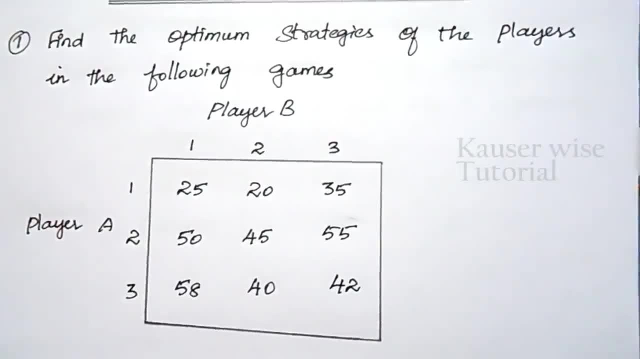 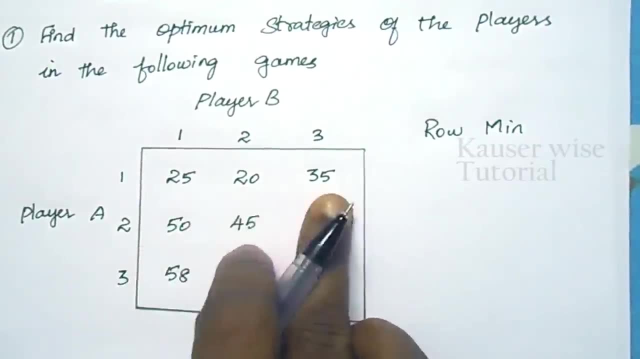 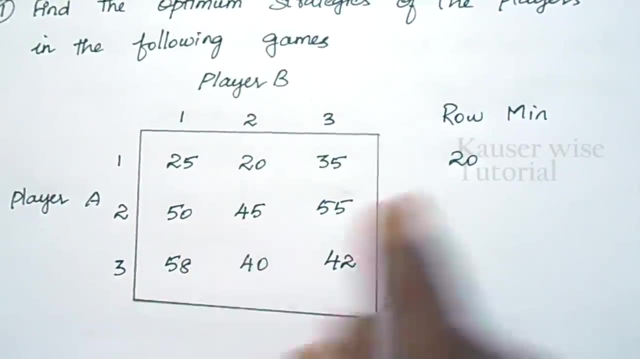 These are the outcome of different combinations. OK, now, first you need to find the row minimum. OK, look at the first row, which is the least value: 20 is the minimum value. So right here, 20. in the second row, minimum value is 45.. In the third row, minimum value is 40.. Now you need to find the column maximum. OK, look at the first column: Maximum value is 58.. Second column: maximum value is 45.. In the third column, maximum value is 55.. So, after finding row minimum and column maximum, now you need to find the maximum of these minimum values. So this is called as maximum value. So we need to find the maximum value. So maximum value means maximum of minimum values. So which one is the highest value? 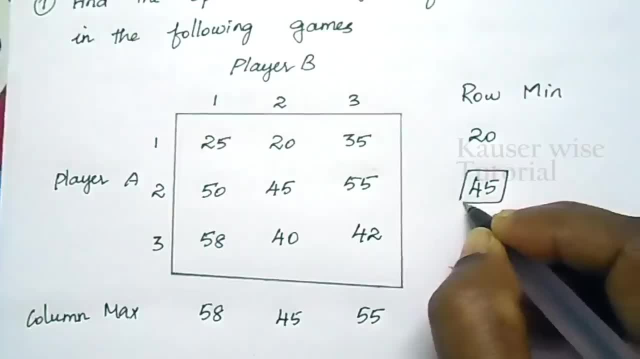 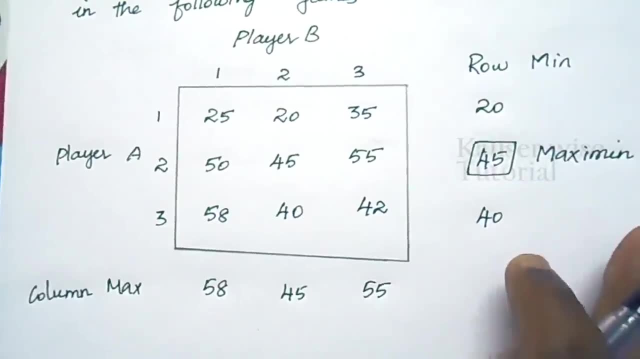 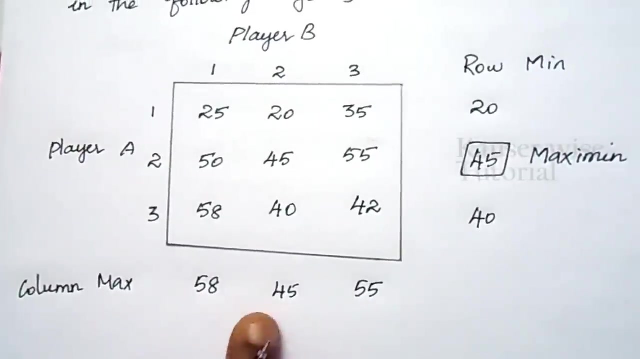 Maximum value 45. So this value is called, OK, maximum value. OK. in the same way, we need to find the minimum value among the maximum. So which is the minimum value among these three values? This one is minimum value. 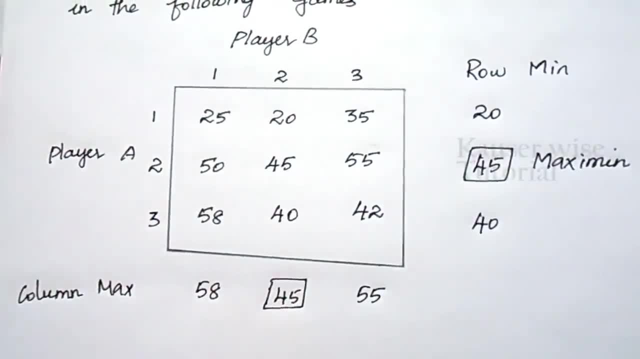 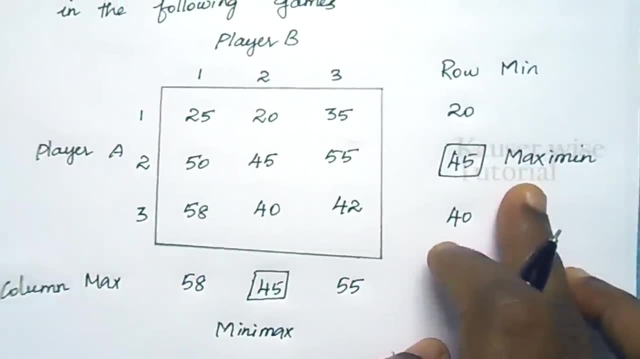 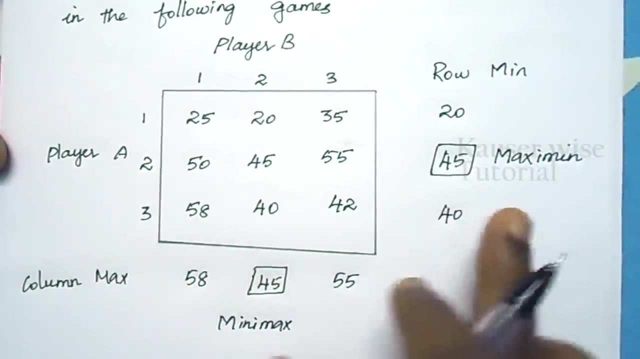 So this is called as minimum value. This one is minimum of maximum value, that is minimax. OK, so this is called as maximian principle and this one is called as minimax principle. As per the pair of matrix, player A is called maximian player and player B is called minimax player. 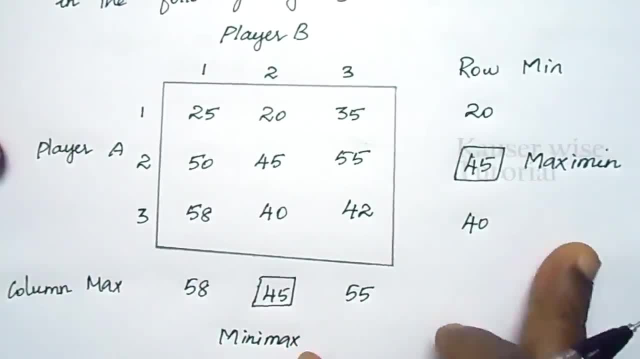 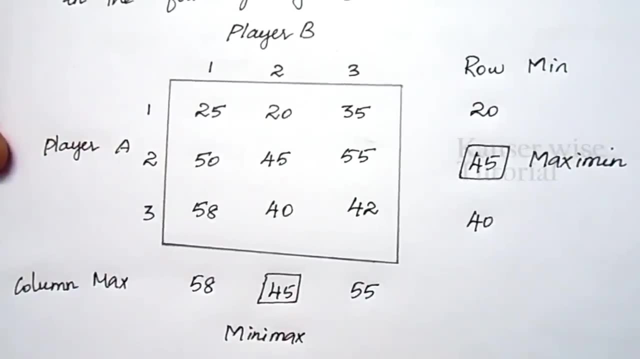 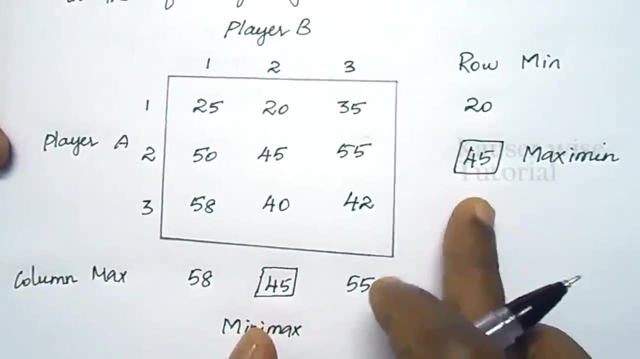 OK, which means player A is maximizing its minimum guaranteed gain and player B is minimizing its maximum loss. OK, so player A is always maximian player and player B is always called as minimax player. OK, so which one is intersecting point? 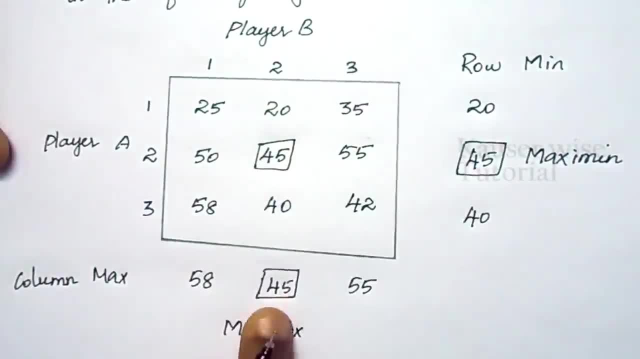 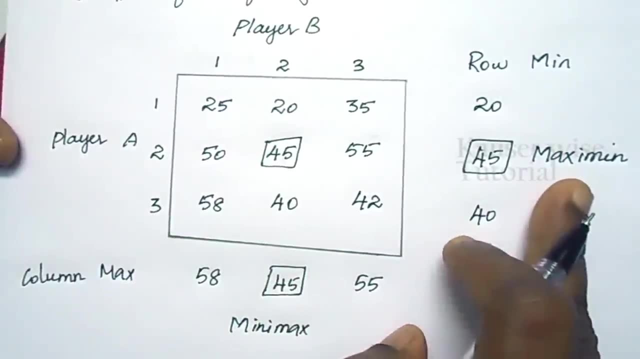 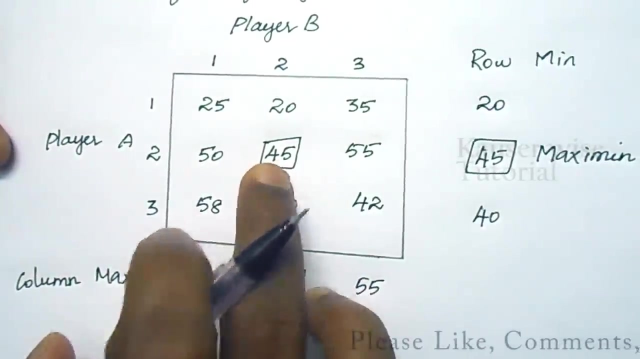 Forty five. Forty five Intersecting point is forty five Now. so this point is called saddle point. OK, because the maximum value is equal to minimax value. So this game has a saddle point. So the value of the game is forty five. 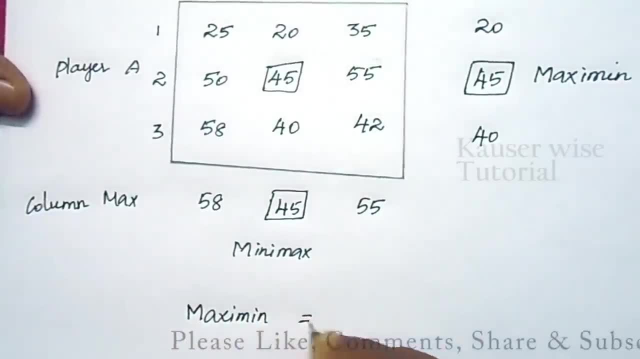 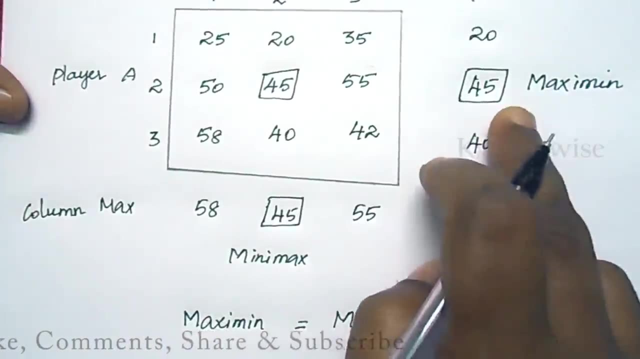 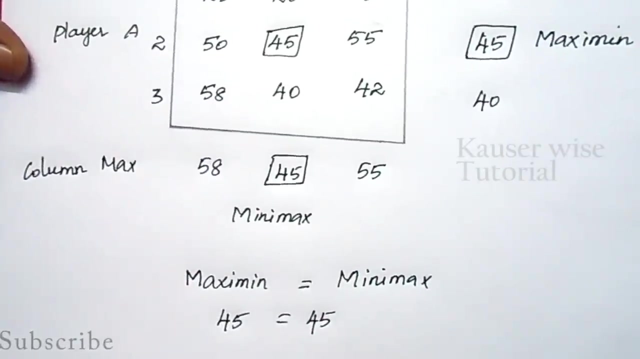 Here the maximum value is equal to minimax value. So this game has saddle point. So maximum value is equal to forty five and minimax value also forty five. So both the values are equal. So this game has saddle point. Now what is the value of the game? 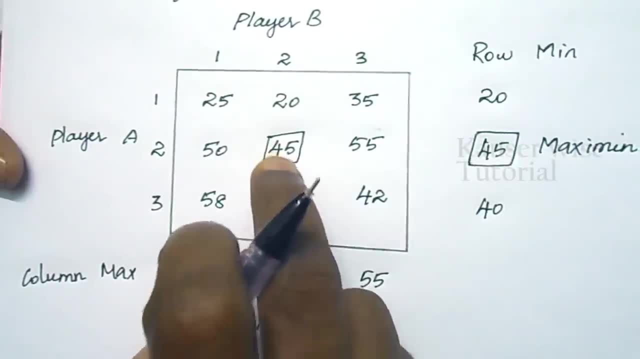 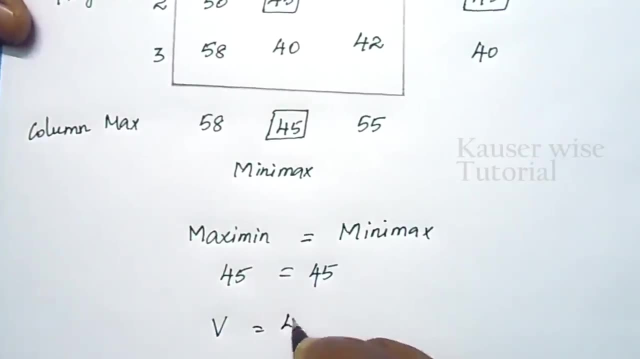 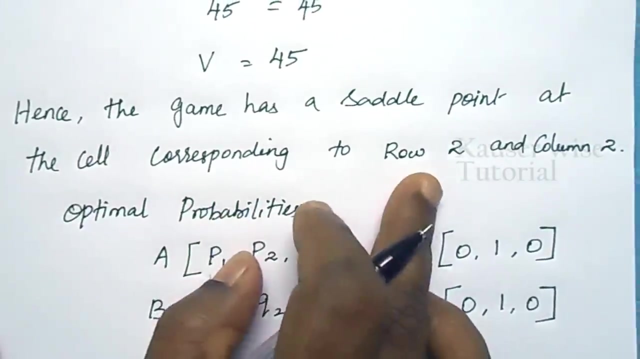 See, the intersecting point is this one. So the value of the game is forty five. So we represent value of the game, So we is equal to forty five. Forty five Hence the game has a saddle point at the cell corresponding to second row and second column. 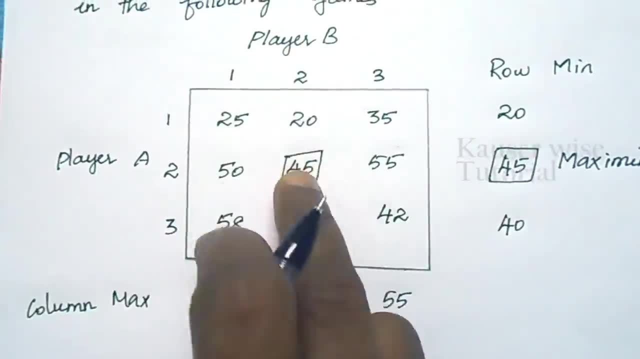 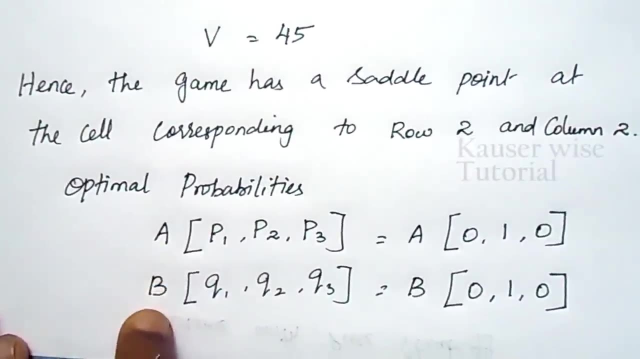 See the matrix, Second row and second column. The value of the game is forty five. OK, see the optimal probabilities of player A and player B. So three strategies are there: P1, P2, P3. for B, Q1, Q2, Q3.. 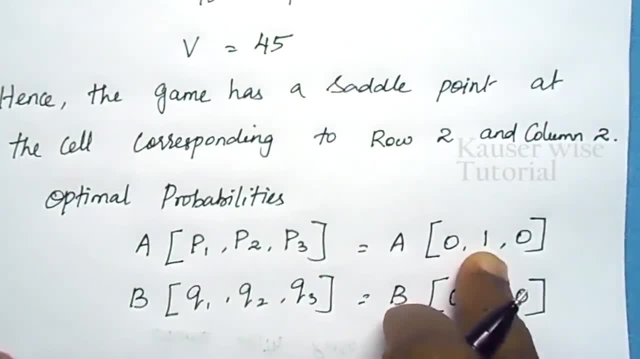 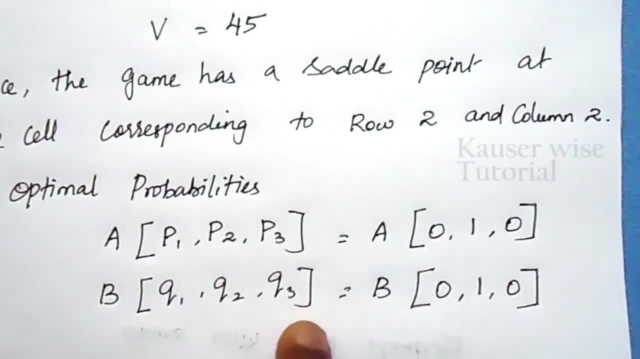 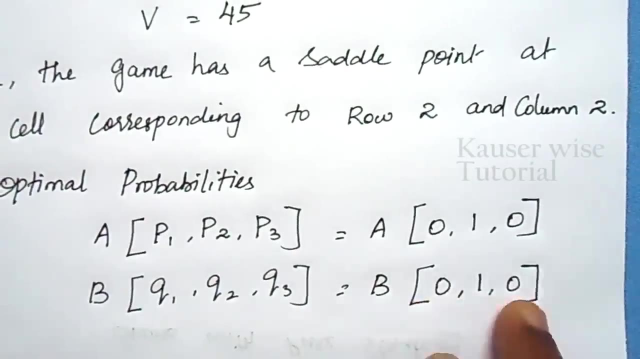 OK, so player A can select the second strategy. The probability is one. The remaining strategies are zero. OK for B also, the optimal probability is: you need to select the second strategy. The probability is one for. the remaining probability is zero. 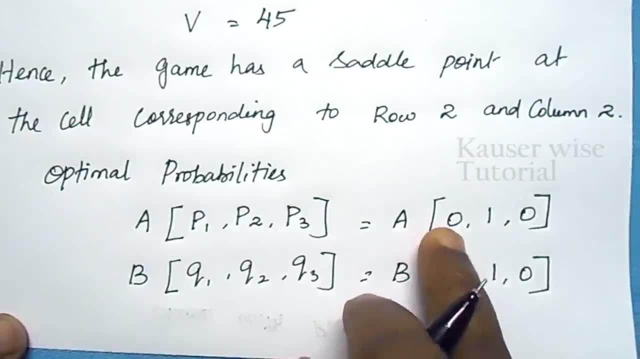 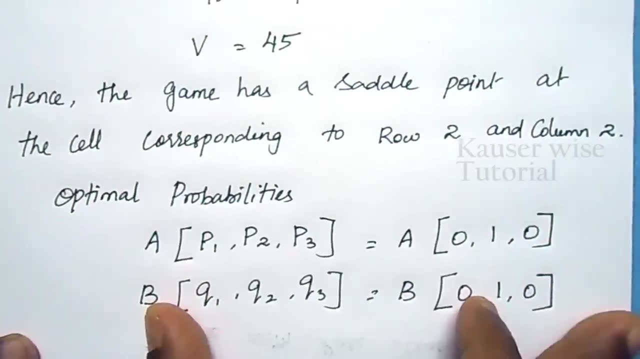 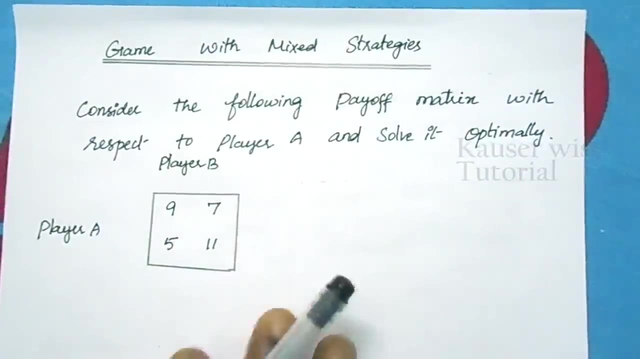 The sum of the probabilities will be equal to one. That is zero plus one plus zero is equal to one, So this game is a pure strategy. Let us see the problem for mixed strategy Now. let us see the game theory with mixed strategy. OK, so here we have one problem for mixed strategy. 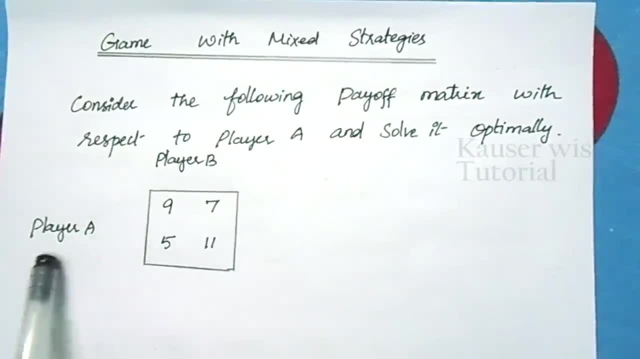 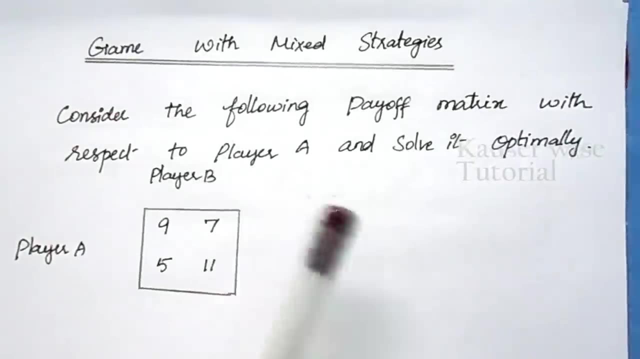 So consider the following: two into two pair of matrix with respect to player A and solve it optimally. OK, so mixed strategy means if a game has no saddle point, then the game is said to have mixed strategy. So what is the meaning of saddle point? 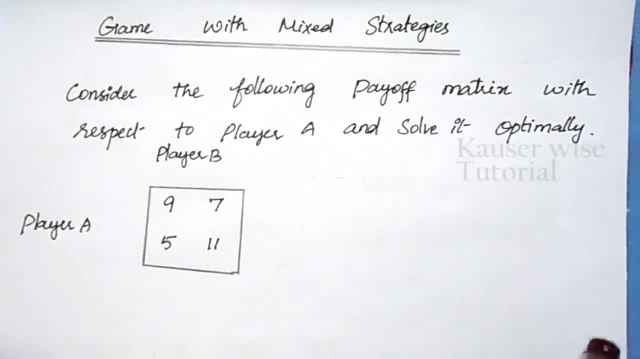 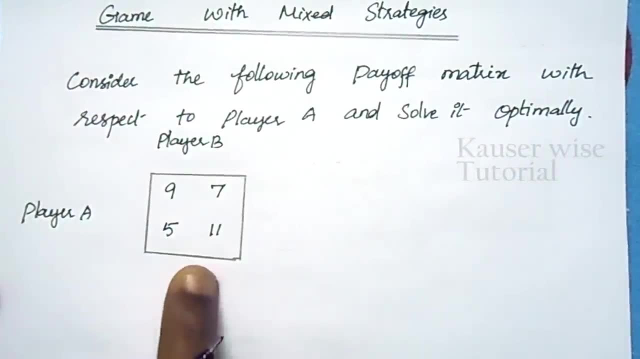 Saddle point means the maximum value is equal to minimax value. If not, then the game will have mixed strategy. Let us confirm whether this game has a saddle point or not. OK, then we can go for the procedure for mixed strategy. 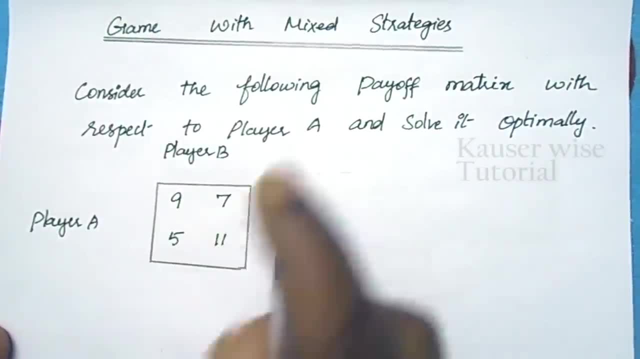 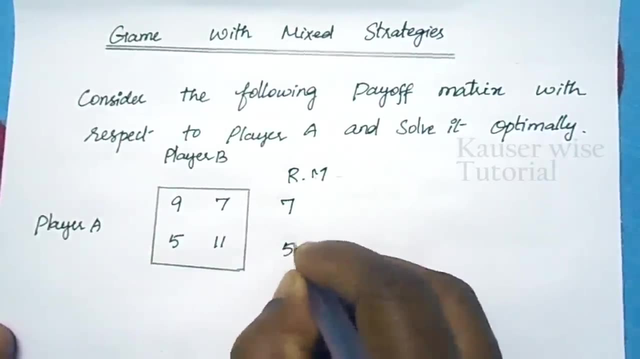 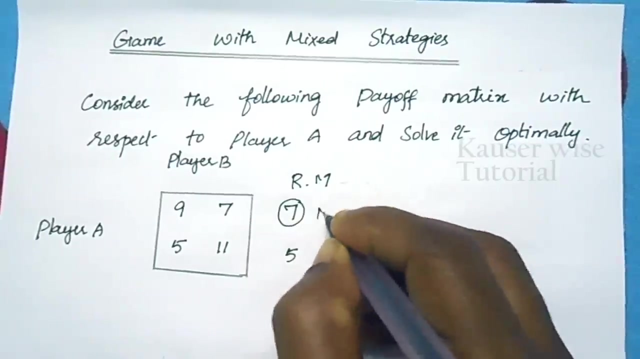 OK, in order to find out the saddle point, find out the row minimum. So row minimum is seven. Here, the row minimum is five. OK, now find out the maximum value. So which one is maximum value? Seven is the maximum value. 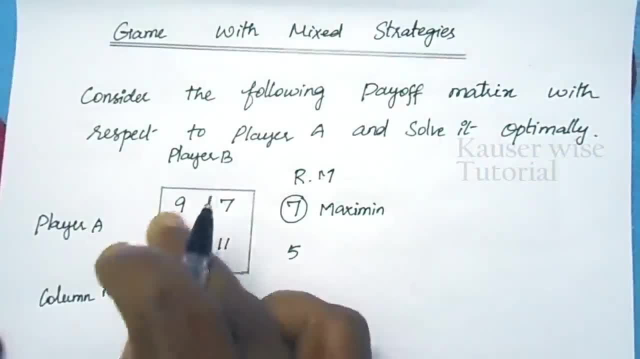 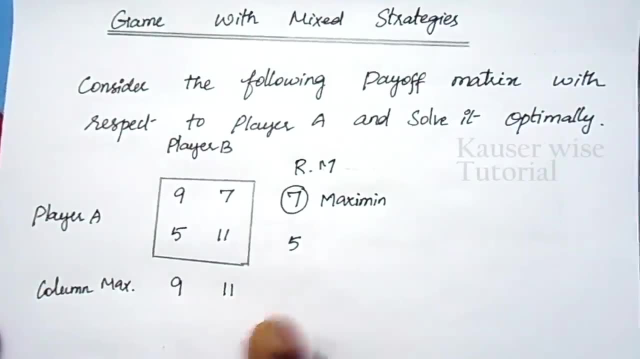 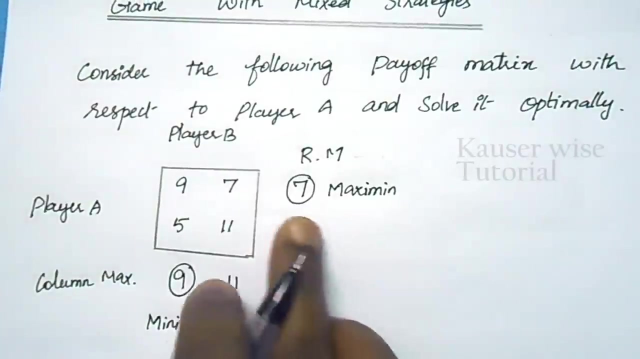 In the same way. find out the column. maximum Maximum value is nine, Here eleven. OK, among these two values, which one is minimum? Nine is the minimum, So this one is minimax value. See, in this problem, the maximum value is not equal to minimax value. 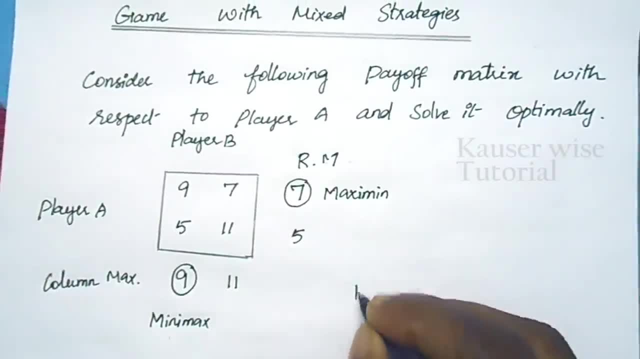 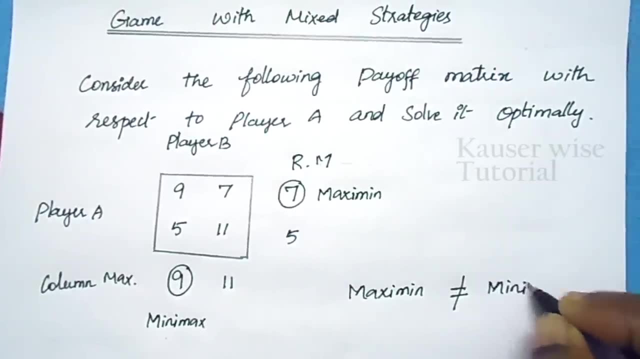 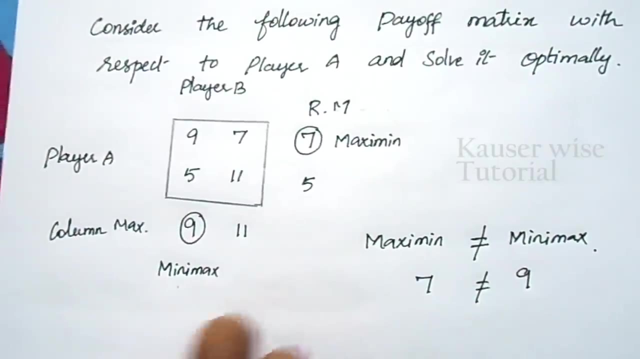 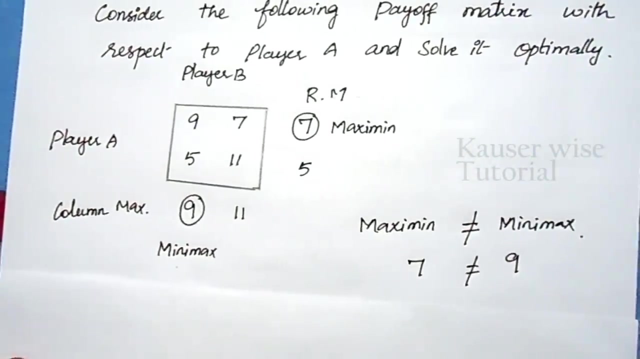 So this game has no saddle point. That is, maximum value is not equal to minimax value. That is, seven is not equal to nine. So this game has no saddle point. Now we'll proceed for mixed strategy. OK, so in order to proceed, mixed strategy- take the two into two pair of matrix. 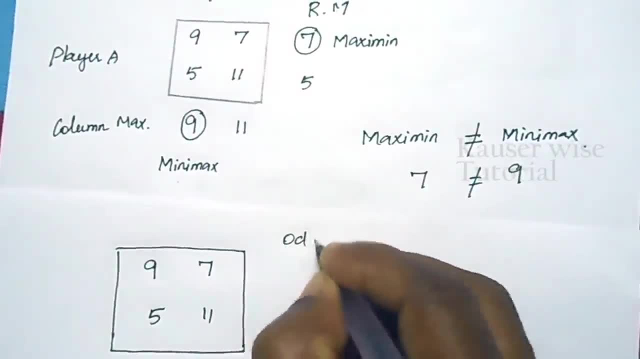 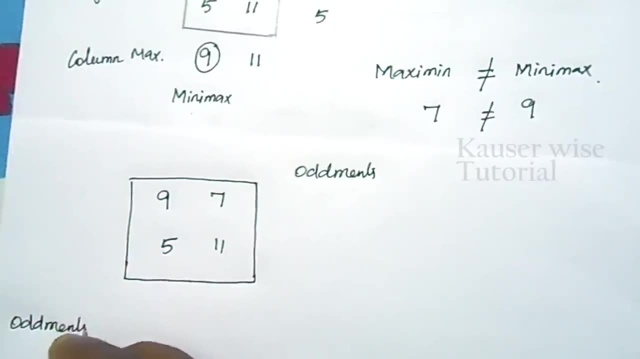 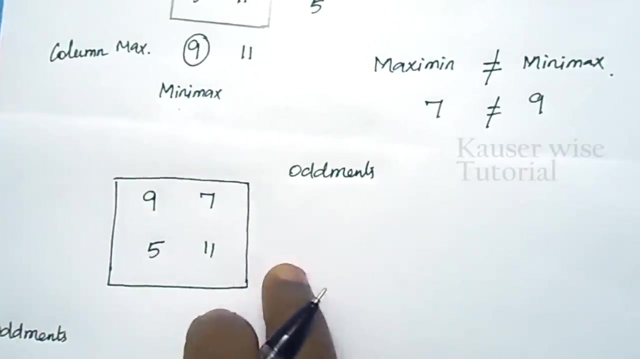 The first step is find out the ordnance for row as well as for column. OK, so ordnance means find out the difference between nine and seven and write it against the second row in the same way, Find out the difference between these two values and write it against first row. 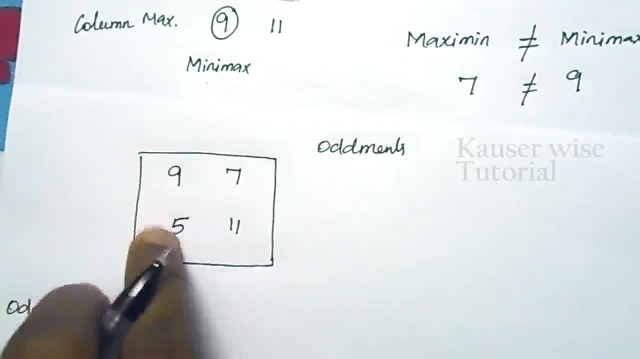 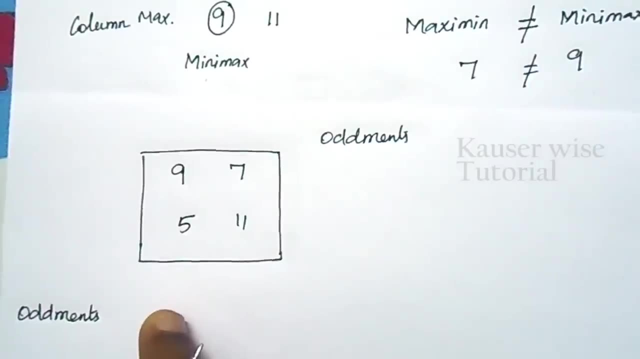 In the same way. do it for column also. So find out the difference between these two values and write it against second column, and difference between these two values and write it against first column. So when you find ordnance, take the highest value first and find out the difference. 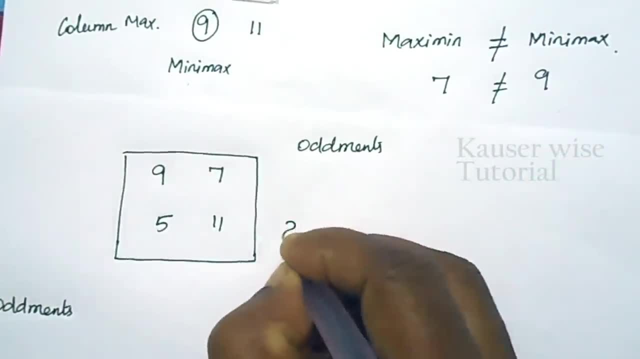 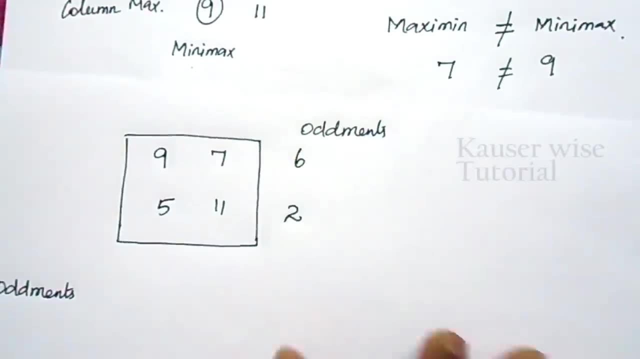 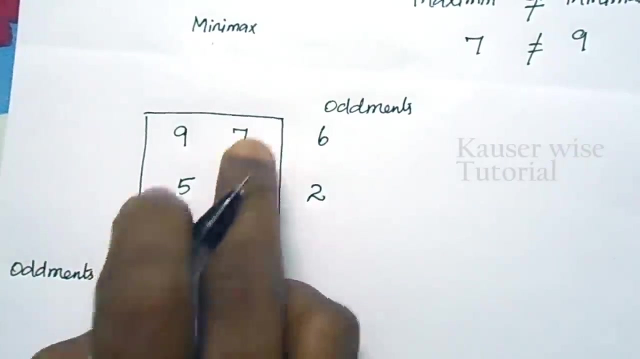 OK, nine minus seven two. write it here. And here highest value is 11, no. so 11 minus five six. Write it against first row. in the same way for column nine minus five four right here Here: 11 minus seven four. write it here. 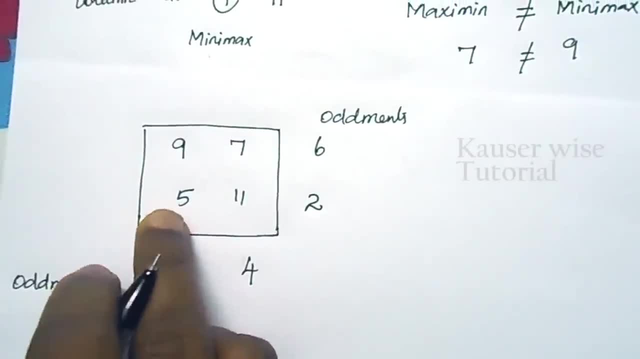 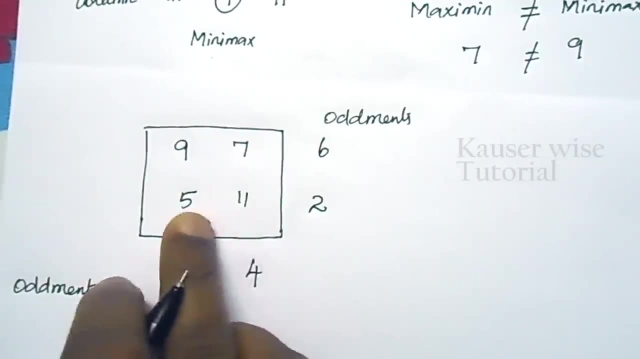 OK. so if we get any negative value, for example five minus eleven, OK, then you have to take the positive value first. So five minus Minus 11, no, so it will be plus 11.. Then the answer will be 16.. 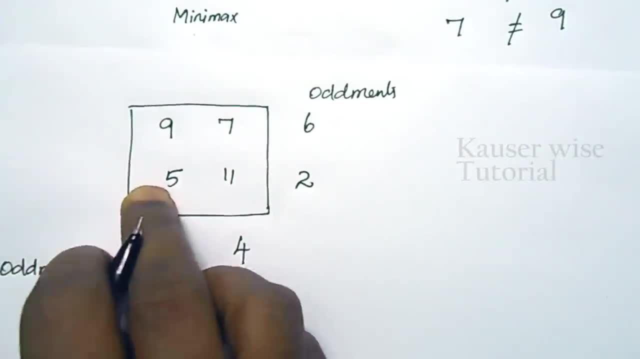 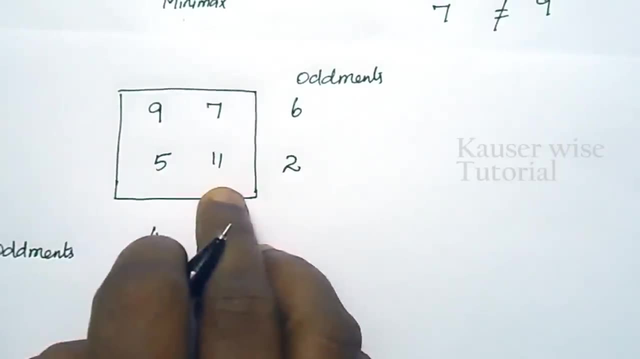 And you have to write 16 here. If you get a minus five, OK, take the highest value first, that is 11.. So 11 minus minus five. no, so plus five. Then the answer will be 16.. Let us see the second step. 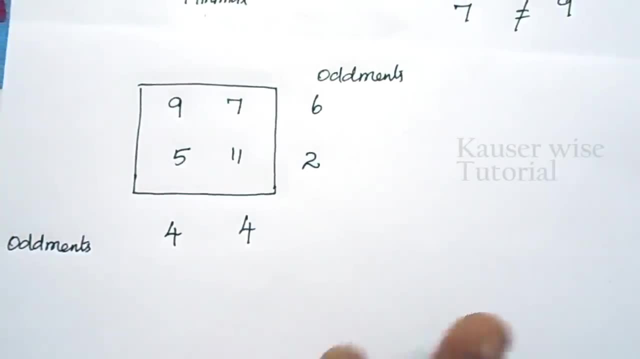 So, after finding the ordnance, the next step is we need to find the probability. OK, for probability there is a formula, but here I'm not going to use any formula. We are going to see a simple procedure to find out the probability. 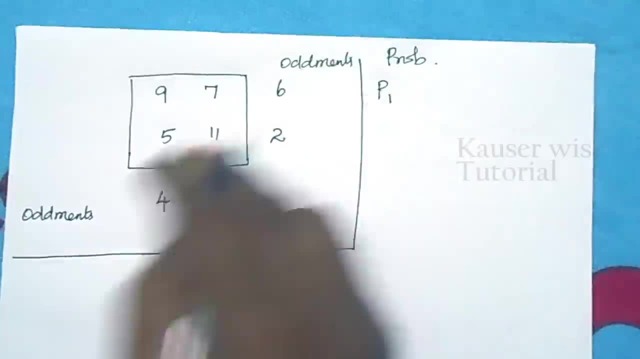 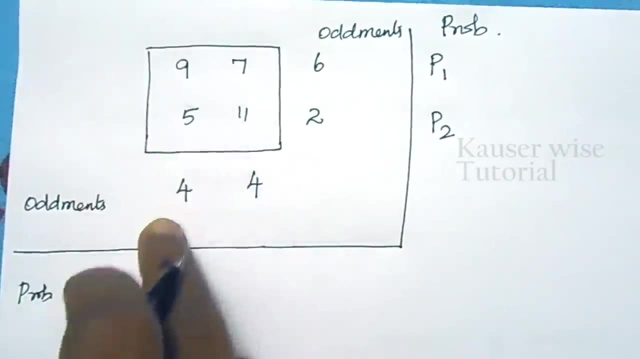 OK, for that, the first row, we need to find P1.. For second row, we need to find P2.. OK, in the same way, we need to find the probability. OK, for the first column, we need to find Q1.. 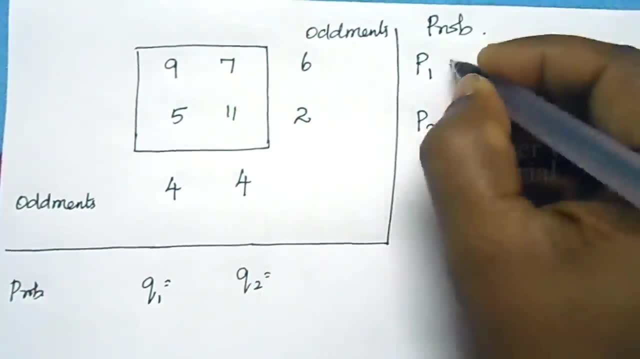 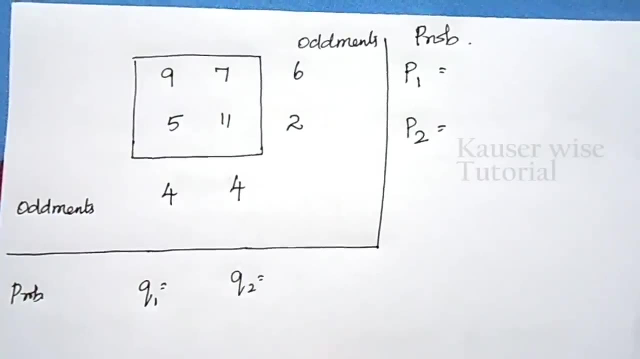 For second column, we need to find Q2.. OK, so there is a formula to find out P1, P2, Q1, Q2.. So here I'm not going to use any formula. We can calculate the P1, P2 and Q1, Q2.. 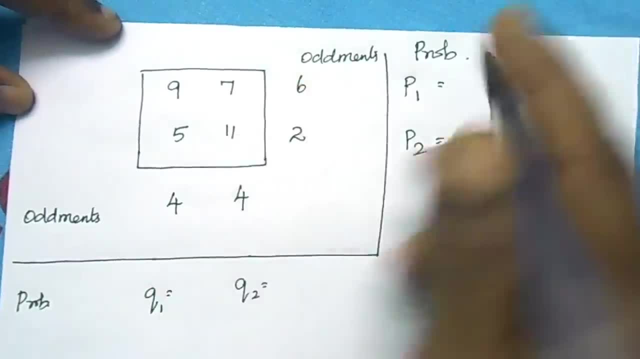 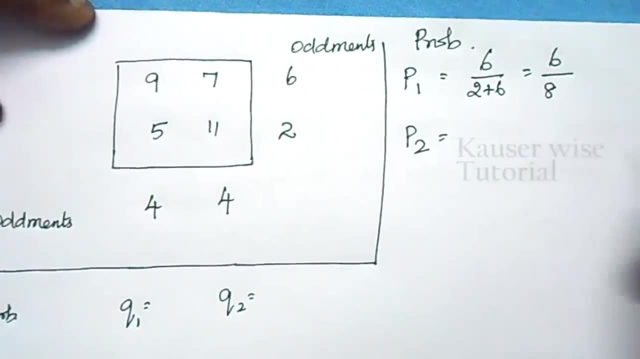 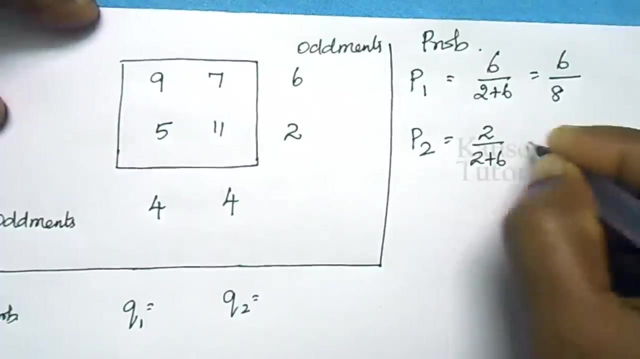 For P1, 6 divided by 2 plus 6.. 6 divided by 2 plus 6 is equal to 6 divided by 8.. OK for P2, 2 divided by 2 plus 6.. 2 divided by 2 plus 6 is equal to 2 divided by 8.. 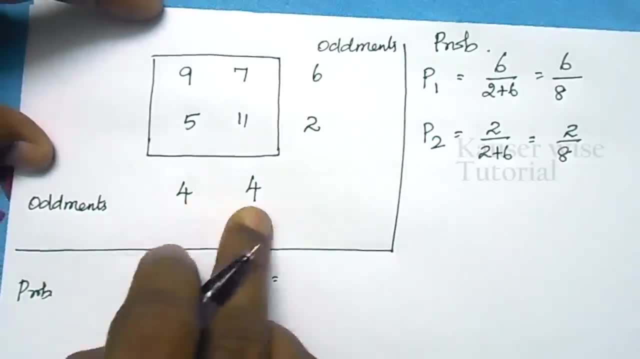 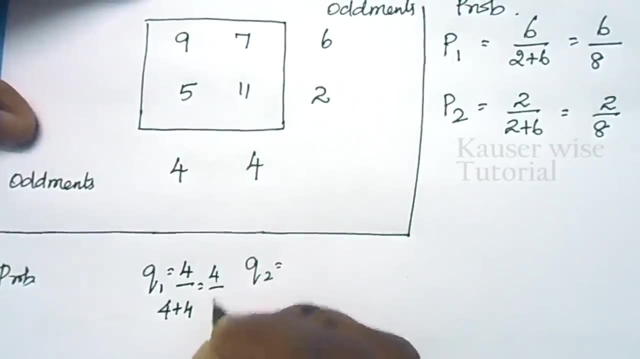 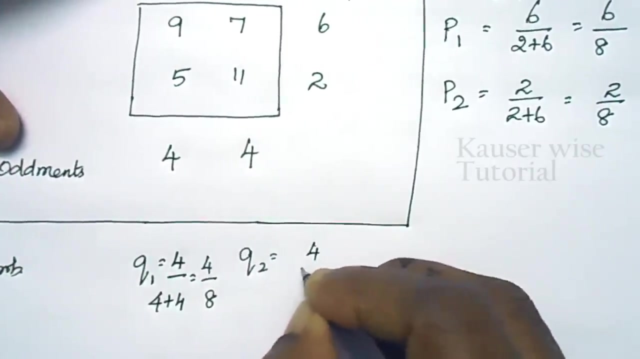 OK, then, for Q1, 4 divided by 4 plus 4.. 4 divided by 4 plus 4 is equal to 4 by 8.. In the same way, for Q2,, 4 divided by 4 plus 4 is equal to 4 by 8.. 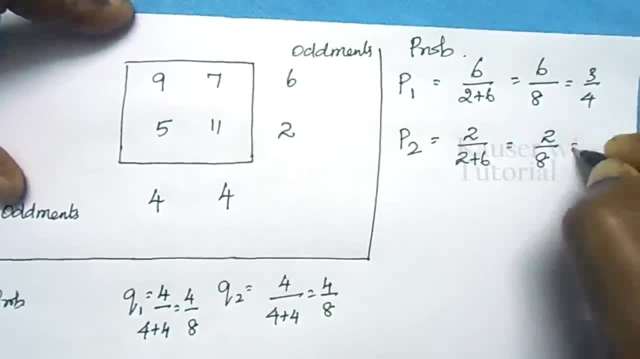 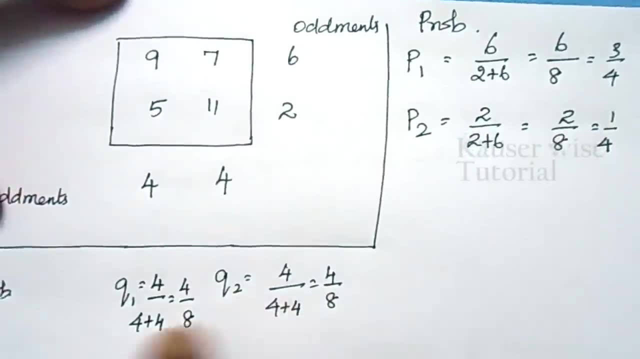 Now simplify: 3 by 4, 1 by 4.. OK, P1 is 3 by 4 and P2 is 1 by 4.. In the same way, Q1, 4 by 8 known, which means 1 by 2.. 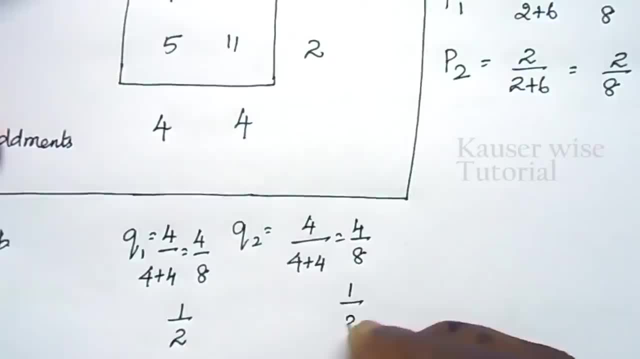 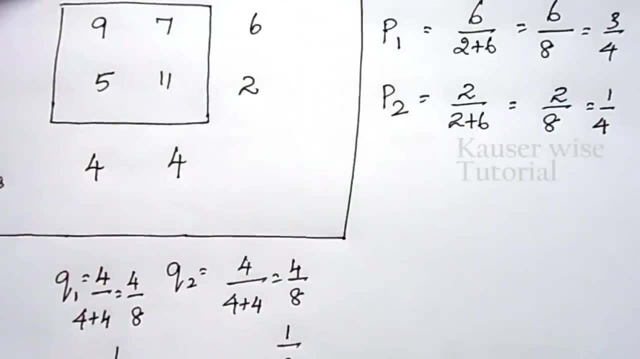 Q2, also 4 by 8 known, so 1 by 2.. OK, P1 value is 3 by 4 and P2 value is 1 by 4.. And Q1 value is 1 by 2 and Q2 value is 1 by 2.. 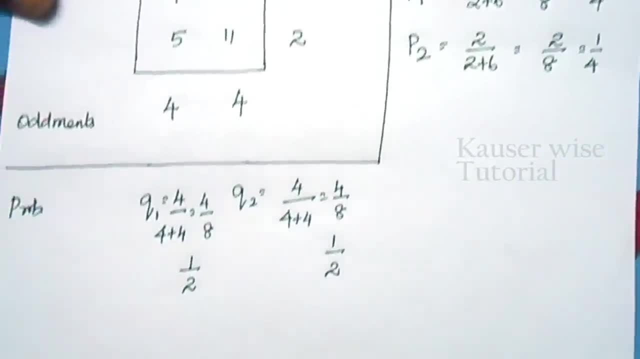 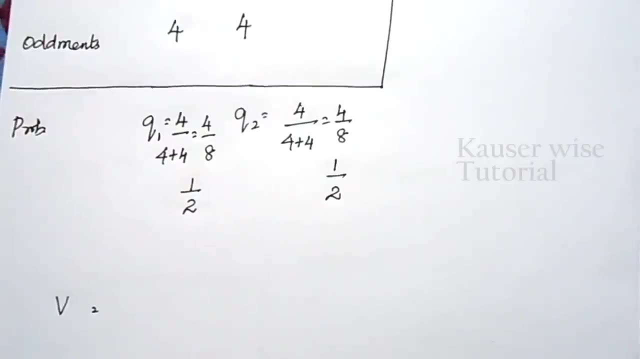 After finding out the probability, now we need to find the value of the game. OK, there are four formulas to find out the value of the game. OK, here I'm not going to use any formula. I'm going to show the simple way to find out the value of the game. 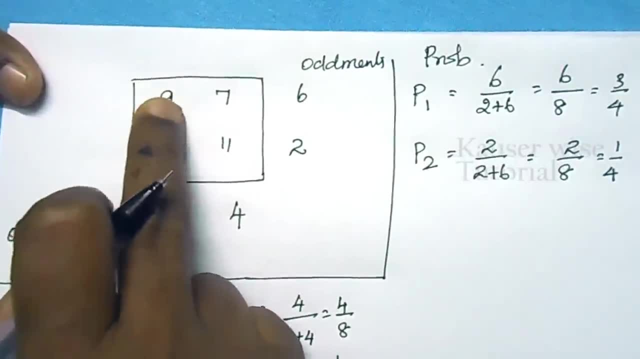 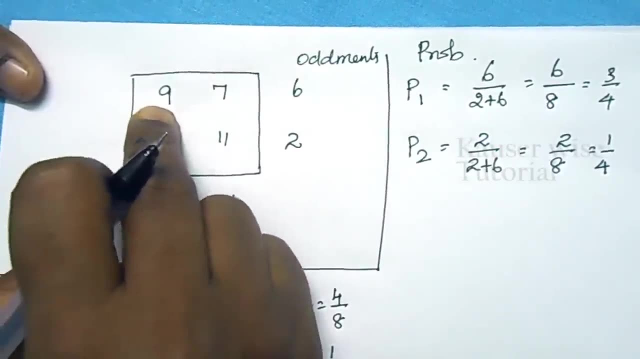 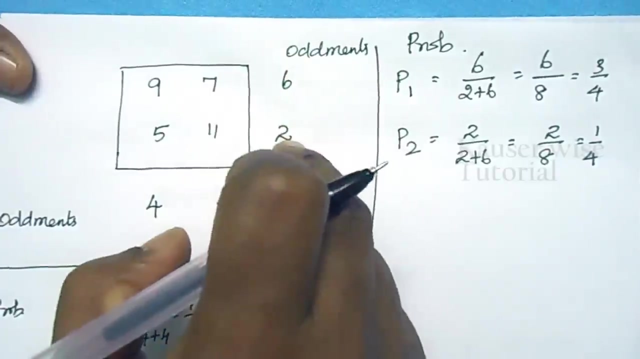 OK, first take the first column value, that is, 9 and 5, and take the ordnance of the first row and second row. OK, so first take the first value, 9 into 6 plus 5, into 2 divided by 6 plus 2.. 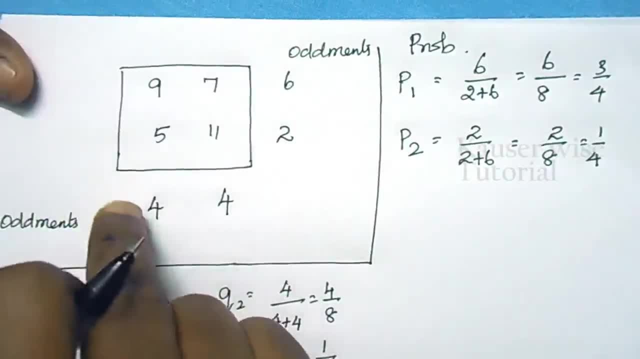 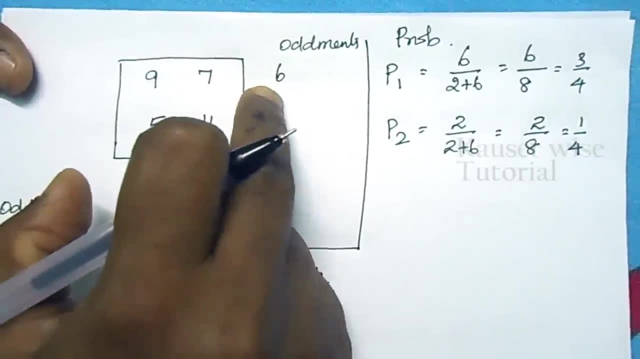 So this is the formula to find out the value. OK, so again I repeat, take the first column value and take the row ordnance, So 9 into 6 plus 5 into 2 divided by 6 plus 2.. 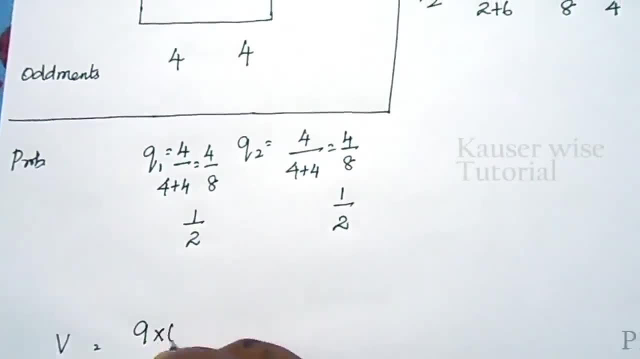 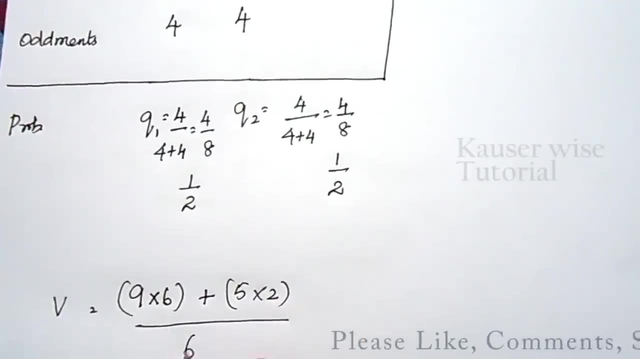 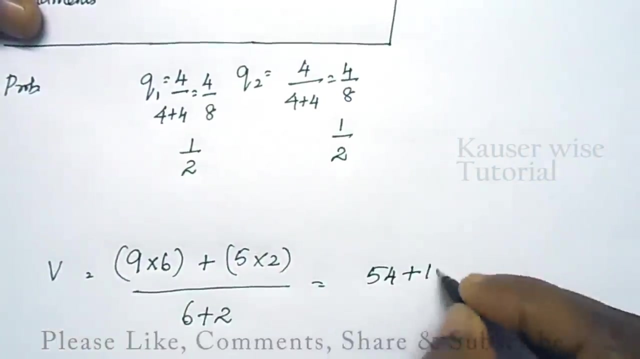 OK, I'll show 9 into 6 plus 5 into 2 divided by 6 plus 2.. OK, 9, 6 are 54 plus 5 into 2, 10 divided by 6 plus 2, 8.. 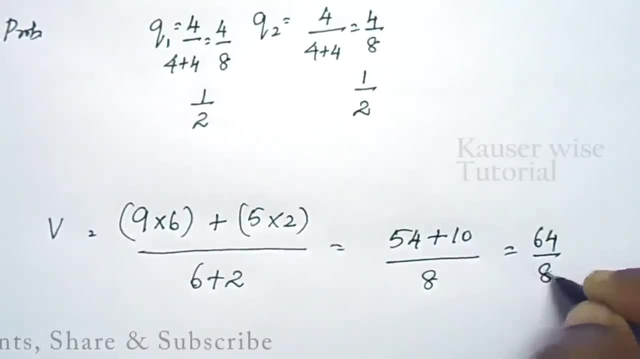 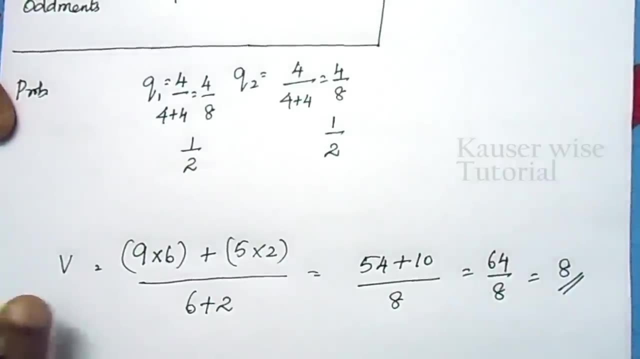 So what is the answer? 64 by 8 is equal to 8.. OK, the value of the game is 8.. Now I'm going to show the other possibilities of finding value of the game. But you'll be getting the same value only. 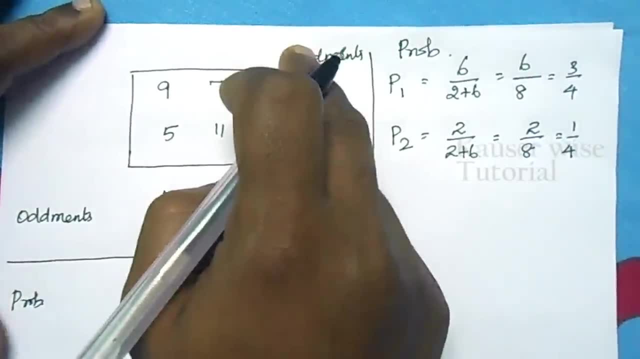 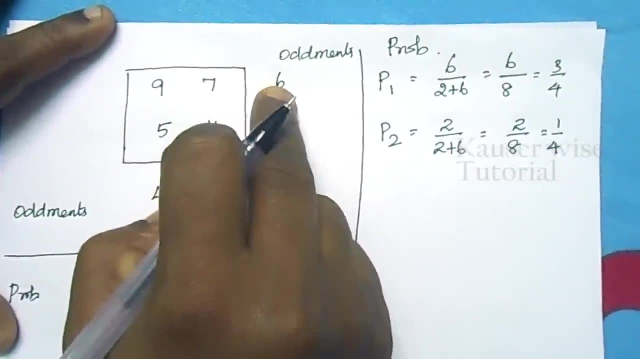 OK, we have taken the first column value and the ordnance of row. If we take the second column, we'll be getting the same answer. Let me show the calculation. See 7 into 6 plus 11 into 2, divided by 6 plus 2, you'll be getting 8 only. 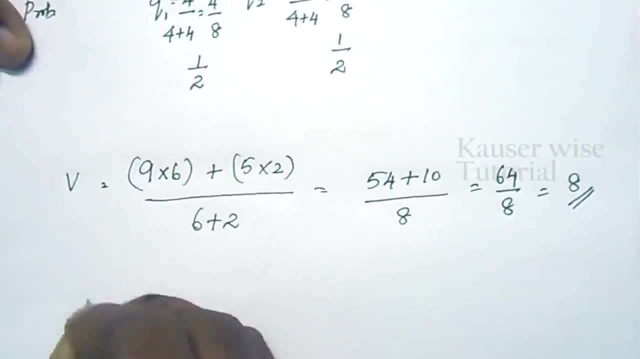 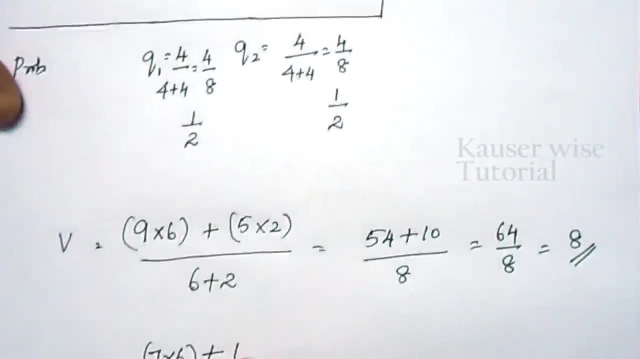 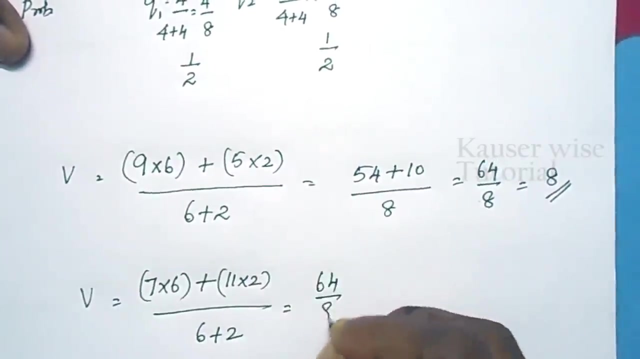 Let me show the calculation: 7 into 6.. 7 into 6.. 6 plus 11 into 2, divided by 6 plus 2.. What is the answer? 64 by 8 is equal to 8.. OK, in the same way, if we take the first two row values. 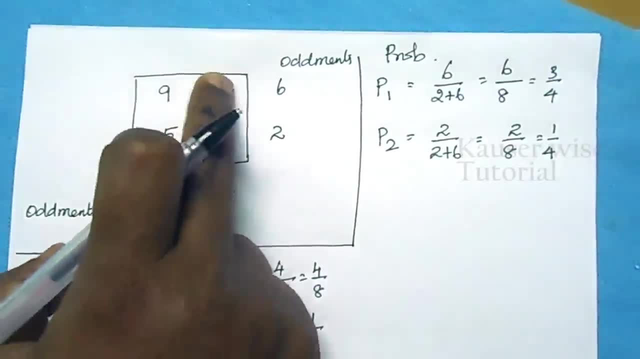 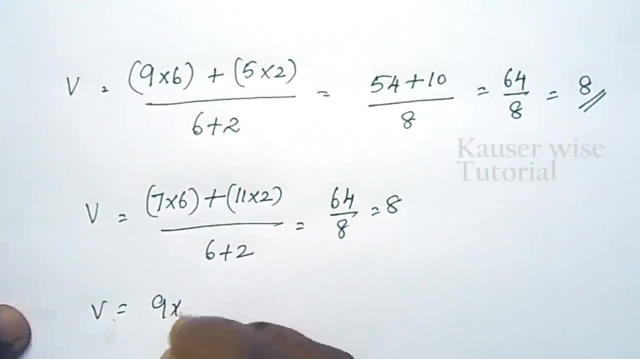 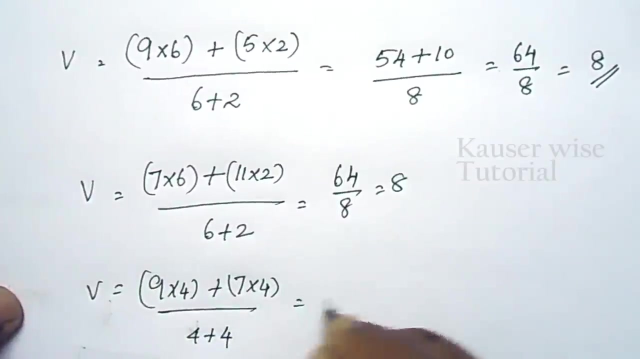 then the value of the game is 9 into 4 plus 7 into 4 divided by 4 plus 4.. Let me show the calculation: 9 into 4 plus 7 into 4.. 7 into 4, divided by 4 plus 4 is equal to 8.. 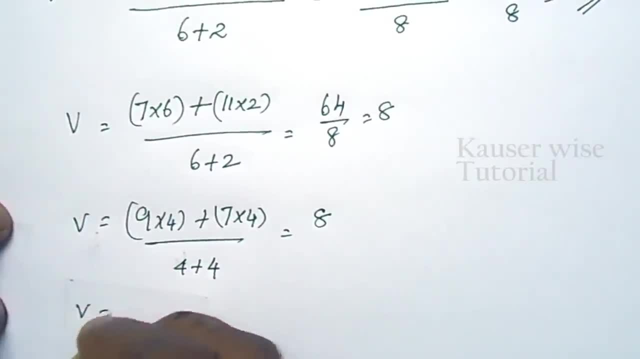 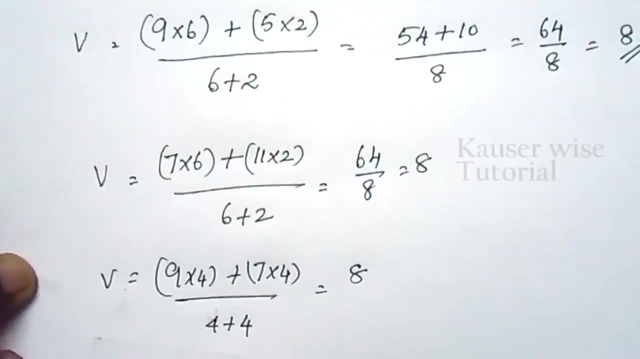 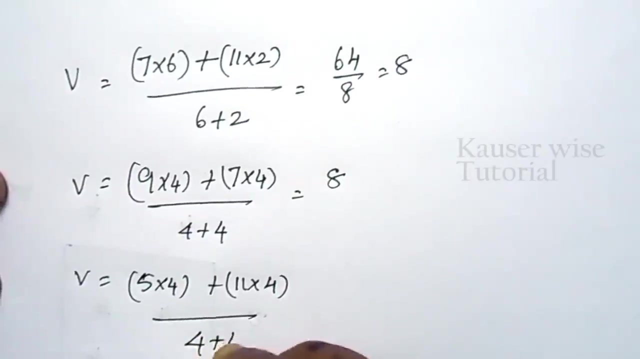 OK, in the same way, the last possibility is 5 into 4 plus 11 into 4 divided by 4 plus 4.. 5 into 4 plus 11 into 4 divided by 4 plus 4, you'll be getting 8 only. 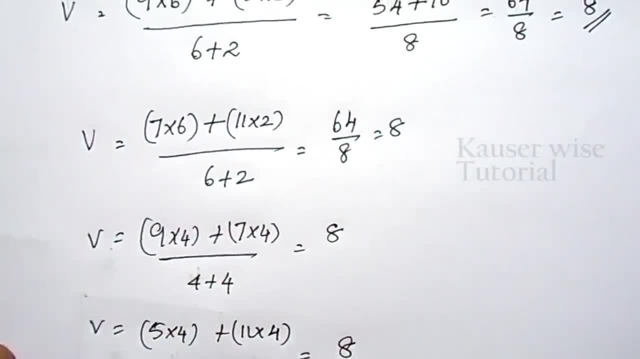 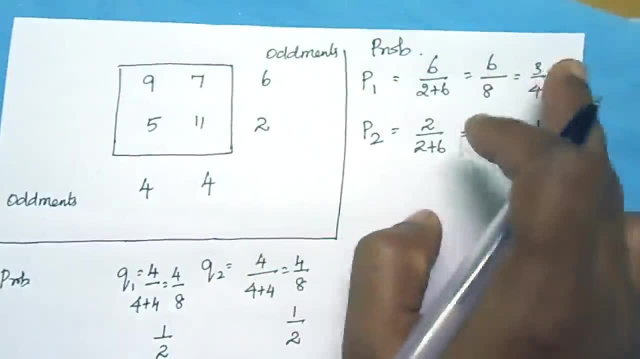 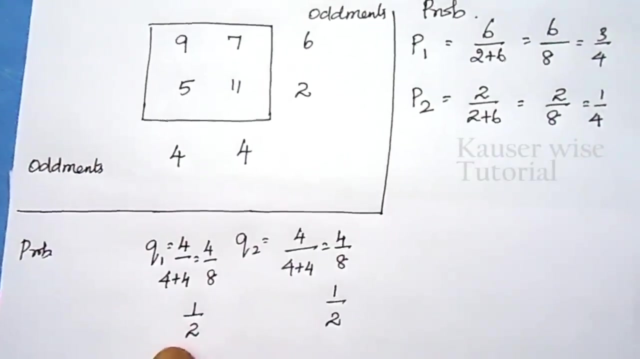 OK, the value of the game will be equal in all the possibilities. Now the final conclusion is: the probability of player A is P1, value is 3 by 4 and P2 value is 1 by 4.. And probability of player B is Q1 value is 1 by 2 and Q2 value is 1 by 2, and value of the game is 8.. 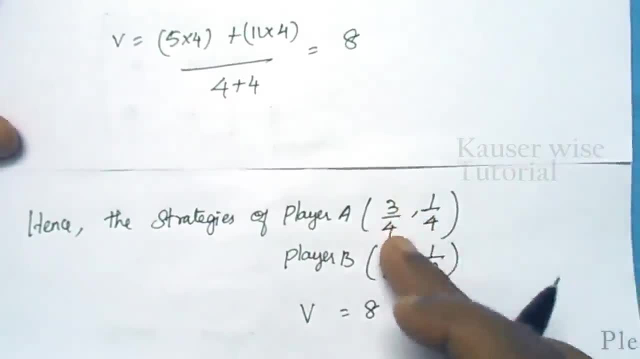 Hence, the strategies of player A is 3 by 4 and 1 by 4. for player B, 1 by 2 and 1 by 2.. And the value of the game is 3 by 4 and 1 by 4. for player B, 1 by 2 and 1 by 2..